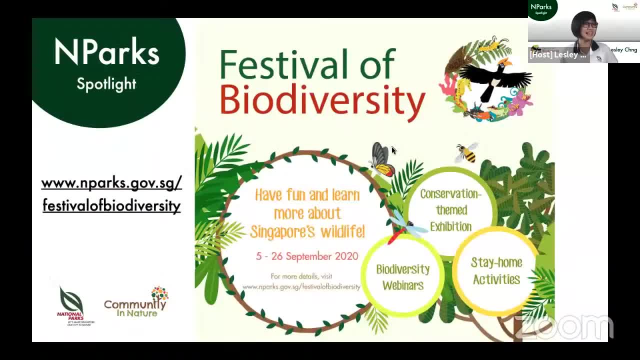 before welcome back, It is now the Festival of Biodiversity, organised by NParks in collaboration with the Biodiversity Roundtable. This is our annual celebration of our national heritage. This year, our festival is online, with several activities from the 5th to the 26th of September. 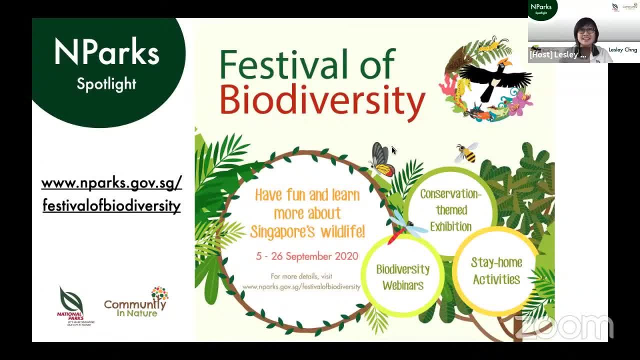 Listen to online talks, download arts and crafts activities or head outdoors to join habitat enhancement sessions or guided walks for small groups. There's lots to do and learn, so check out our website nparksgovsg slash Festival of Biodiversity for more details This month's. 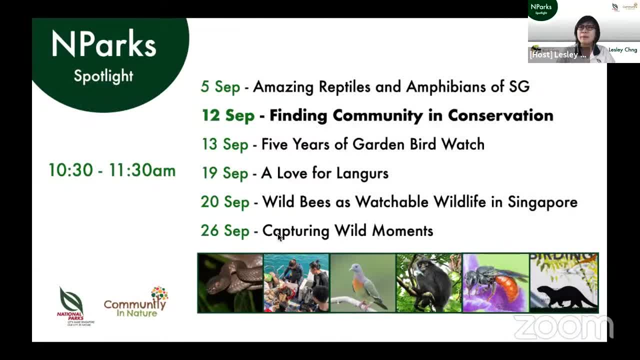 special edition of NParks Spotlight will feature our partners from the biodiversity community. We are online every weekend from 10.30 to 11.30 in the morning, so be sure to join us on Zoom or YouTube. Today we'll be hearing from an active volunteer from Friends of Marine Park. Tomorrow, 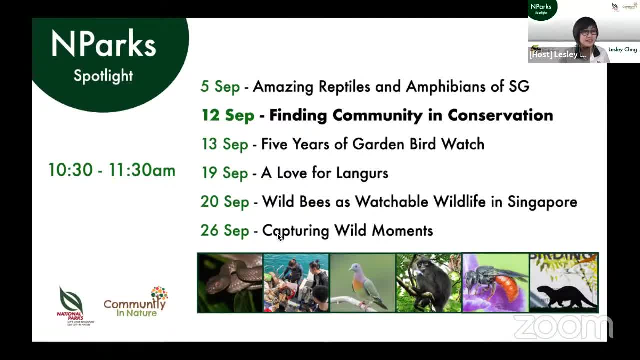 we'll learn about the great work that our citizen scientists have done as part of the Garden Bird Watch programme, And over the coming weeks we'll be joined by our friends from the Raffles Banded Langer Working Group, National University of Singapore and Otter Working Group. 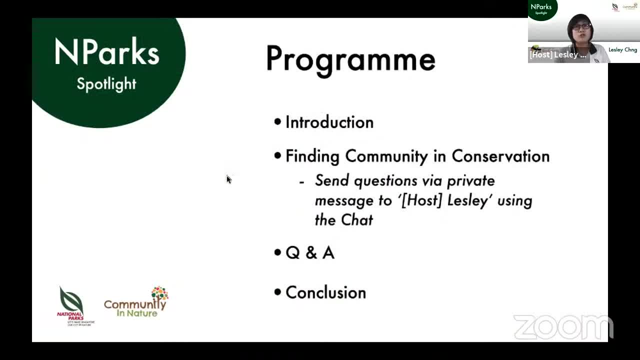 Here is an overview of today's session For those on Zoom. if you have any questions during the talk, please send them to me, Lesley, as a private message using the chat, And we'll try to address a few of them later on. And now let's give a warm welcome to Sam. 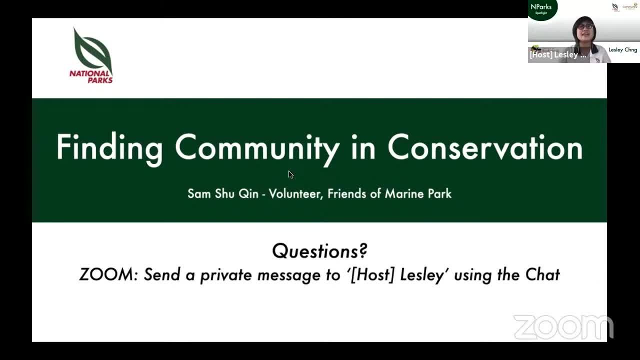 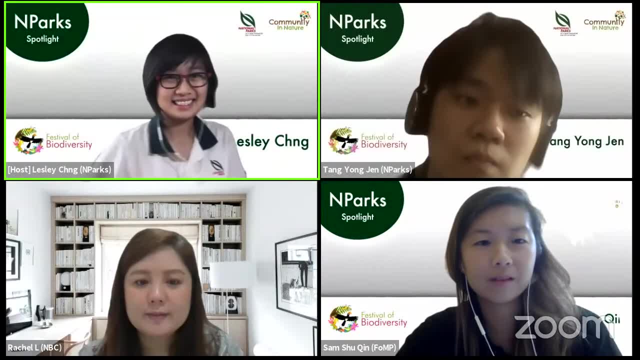 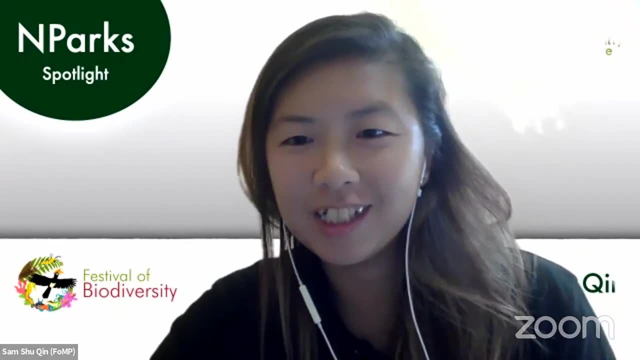 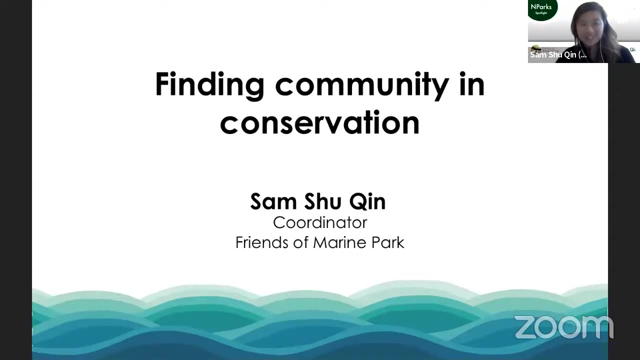 Shu-Tin, from Friends of Marine Park, presenting Finding Community in Conservation. Take it away, Sam. okay, let me do this. hi, can you hear me? yes, we can. okay, great, so hi everyone. thank you, Leslie, for the introduction. I am Sam, and for today's session I will be sharing my experience as a youth volunteer. 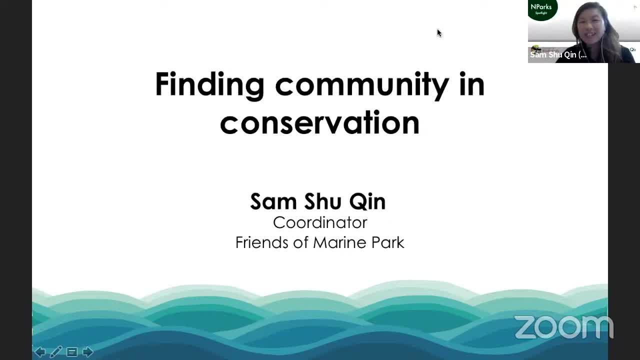 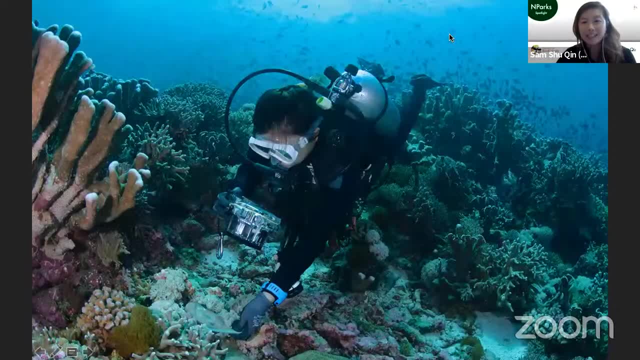 at the Friends of Marine Park community, and I also apologize if I happen to fade in and out of the screen. okay, so here's a little about me. I am a coral scientist at the at the Tropical Marine Science Institute, National University of Singapore, and my research actually focused on 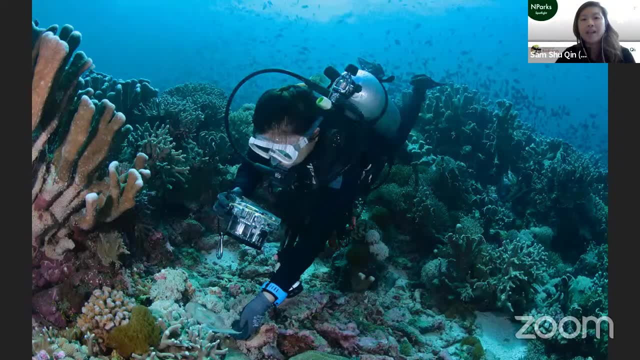 understanding how corals respond to the impacts of coastal development and climate change, so we are also working on developing coral restoration strategies that are best suited for our marine environment. so I spent a lot of time on the research on coral restoration strategies and underwater assessing reef health and checking out coral transplants- and this photo, of course. 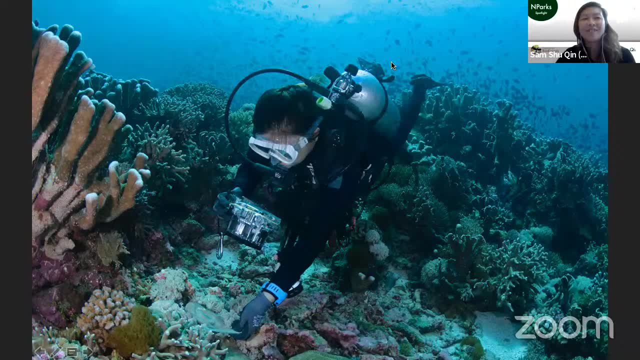 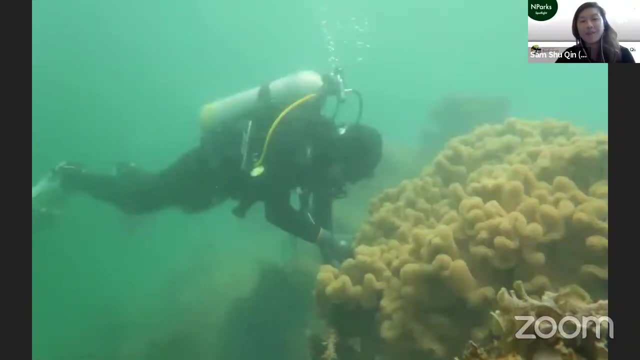 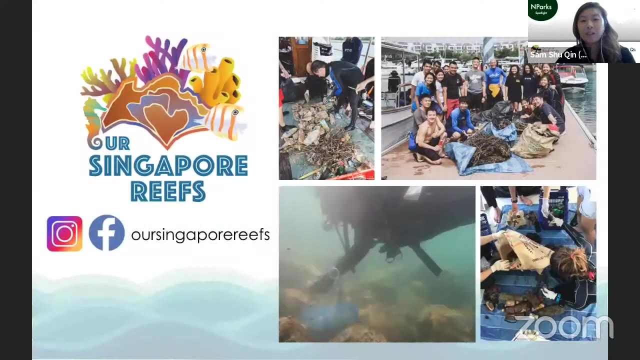 is was not taken in Singapore. okay, this was taken in Raja Ampat, all diverse dream destination, and this is Singapore, and this is actually one of the best days that I have recent- I think it was just last month, okay, so I am also the co-founder of our Singapore reef community. 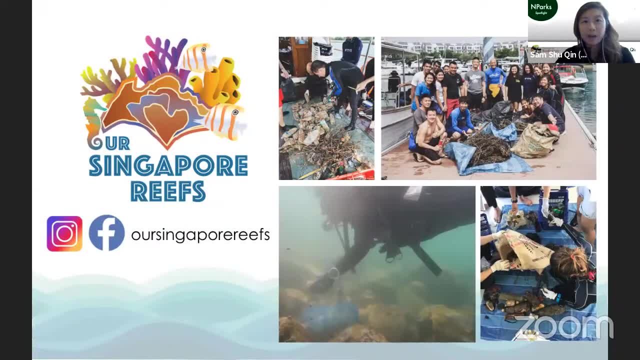 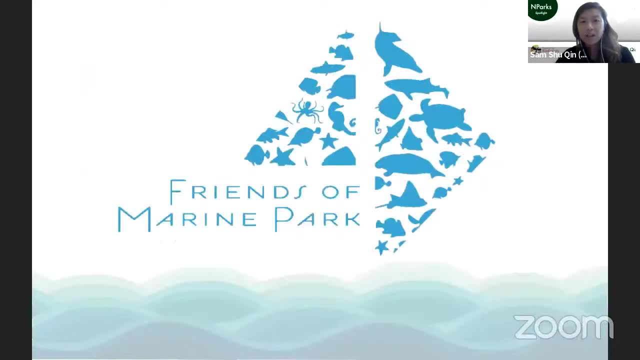 initiative that aims to promote awareness on Singapore's marine biodiversity impacts of marine debris through dive cleanups and educational outreach activities. and because of my involvement in both marine science and public engagement, I am also part of the Friends of Marine Park community, so the Friends of Marine Park community was initiated by Mr Desmond Lee back. 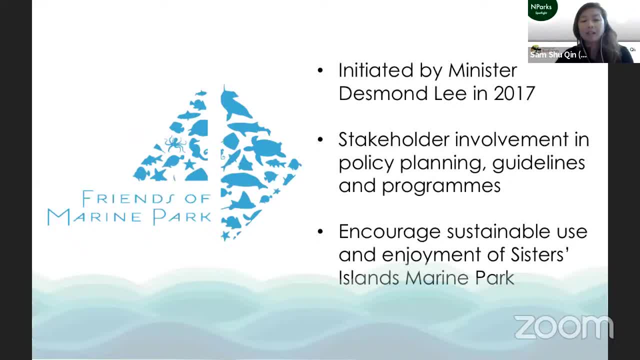 in 2017 to bring different users of Marine Park together and involve them as stakeholders in policy planning, coming up with guidelines and public engagement programs for Sisters Islands to encourage more sustainable use and enjoyment of the park. so this unique network is administrated by Ann Parks and supported by the Ministry of National Development. 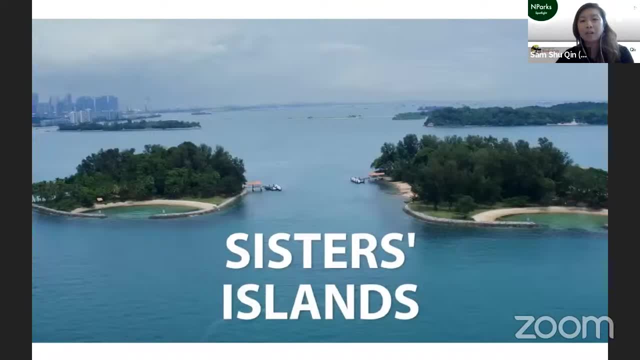 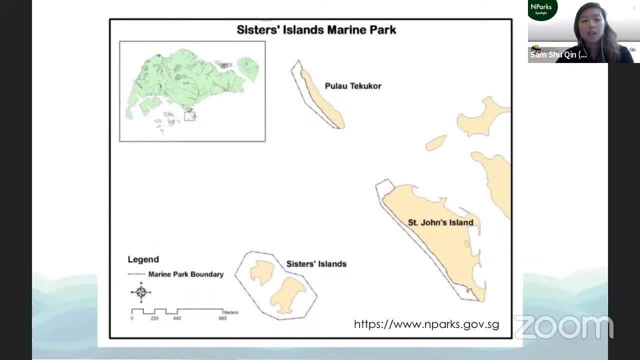 so before I go into more details, let me share a bit more about our first Marine Park. so the Sisters Islands Marine Park expands about 40 hectares around Sisters Islands and along the western Reeves of St john Islands and Pulau Telku Kor ". so the big Sisters Island is open to public seven to seven every day and all other areas under the. 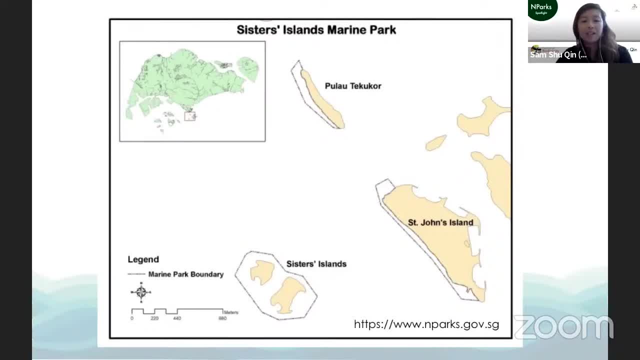 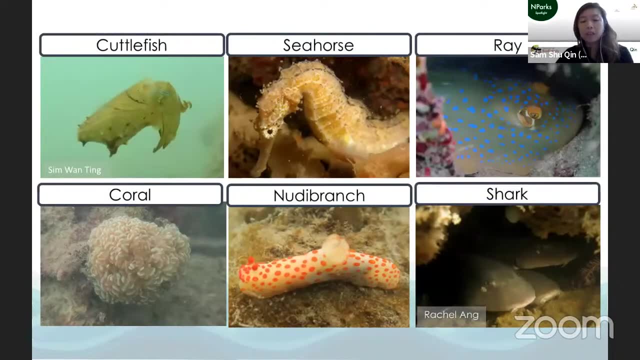 ryves of St john Island and Pulau Telku Kor are 53 hectares of monde, so why does the Bay utmost of the good feel of the'm parole? areas within the marine park are strictly for conservation and research, so this area was selected as a conservation site because of the variety of habitats, including coral, reef, sandy. 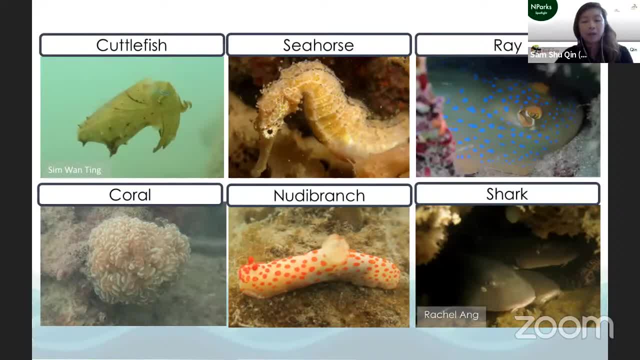 shores, seagrass, meadows and the rich marine biodiversity within the waters. so these are some of the animals we see pretty often while diving in our waters. so we have cuttlefish, we have seahorses, rays, corals, a lot of newly brown and even sharks. so well, if you're lucky, you can. 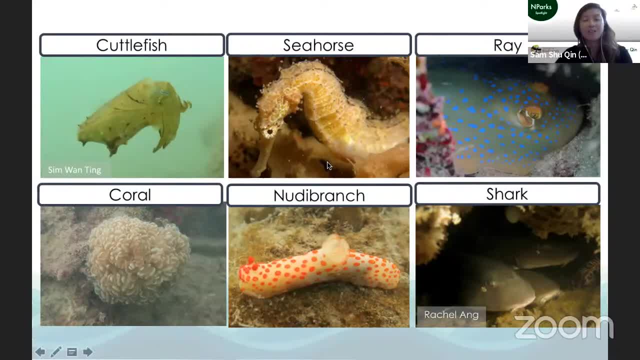 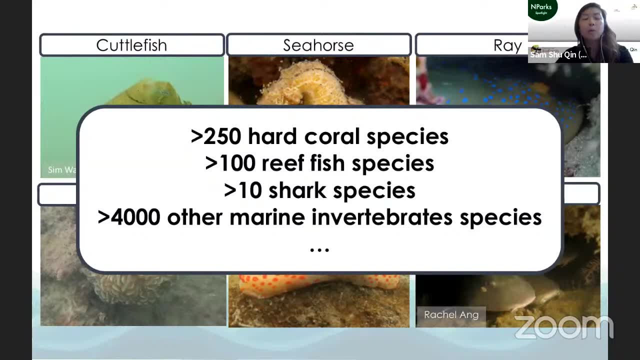 even spot a turtle or pink dolphin along your on your way to the southern islands. okay, so, historically, we have recorded more than 250 coral species. that is almost one third of the entire coral species in the world. so, sisters, islands is also. they are also regarded as a mother reef. 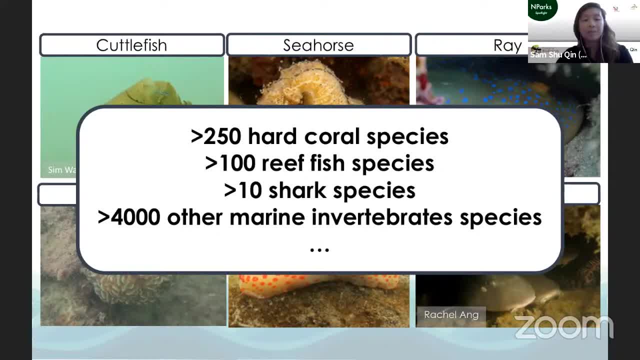 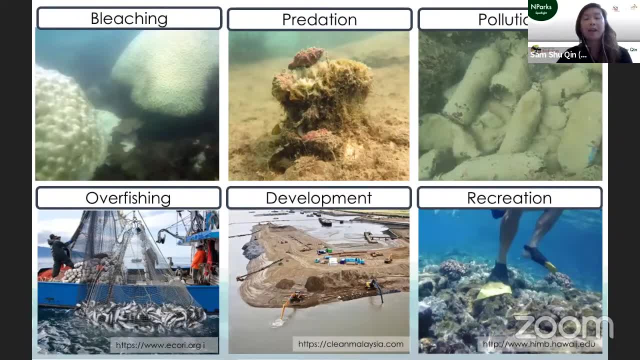 because of the strategic location that it can seed and supply coral larvae to other reefs. so our coastal habitats, such as coral reef, are impacted by natural stresses such as predation, coastal development, unsustainable fishing methods and irresponsible diving habits, and also together with the slow growth and self-recovery of corals. they can- they cannot keep up with scientists. 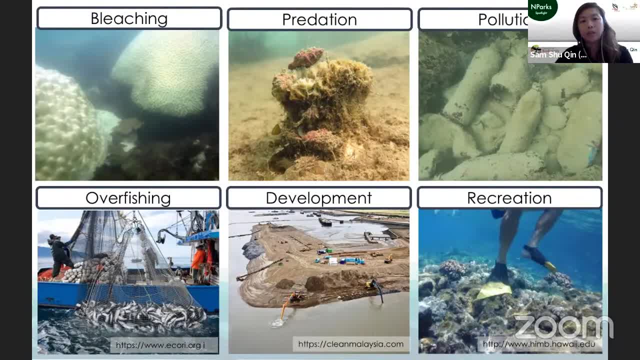 predictions of strongest intensity and this increased frequencies of thermal stress events. so without our intervention in reef recovery, we can potentially lose the ecosystem that can support a lot, a lot of people. so sisters island marine park is a no-take zone, meaning no fishing is allowed there. so it's definitely a good start for us. so with good 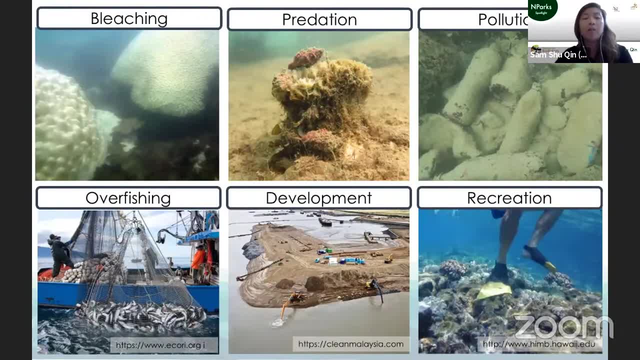 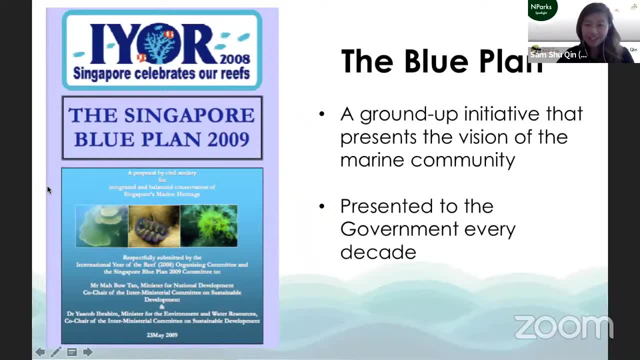 management and responsible use of the area. the marine park can protect and support the precious marine life that we have. and i want to introduce you to the blue plant. so the blue plant is a ground initiative that presents a vision of the marine community and this document that is put 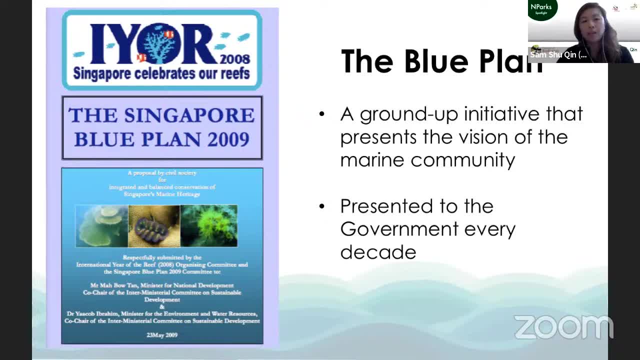 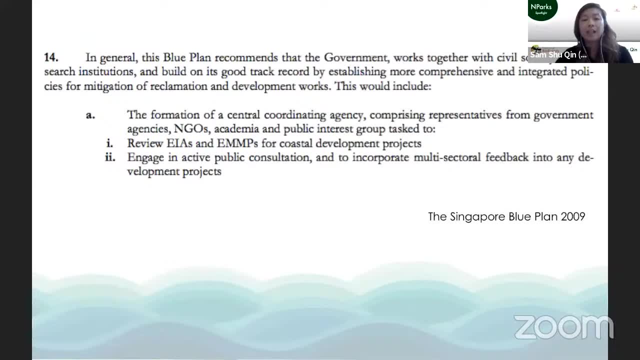 together by the team is presented to the government every 10 years, and in the singapore blue plan 2009, the second, which is the second installment of the blue plan, the community recommended that the government should work together more with civil society and the researchers to establish 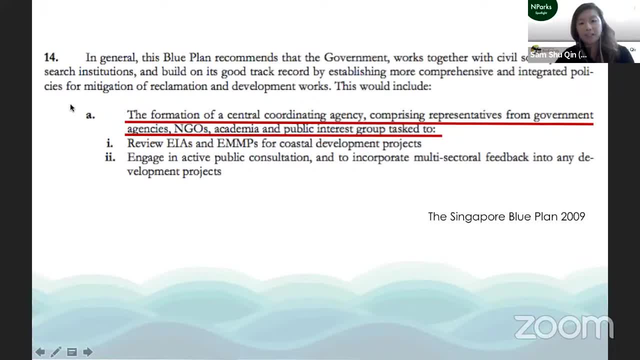 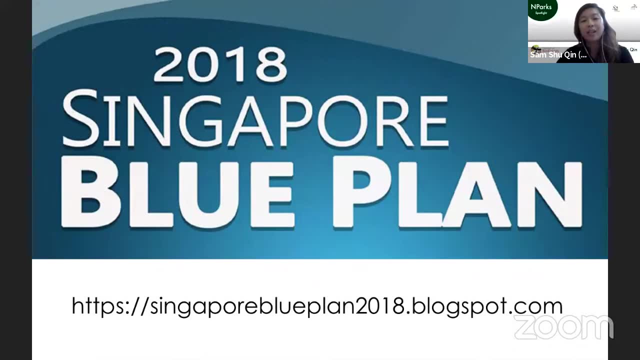 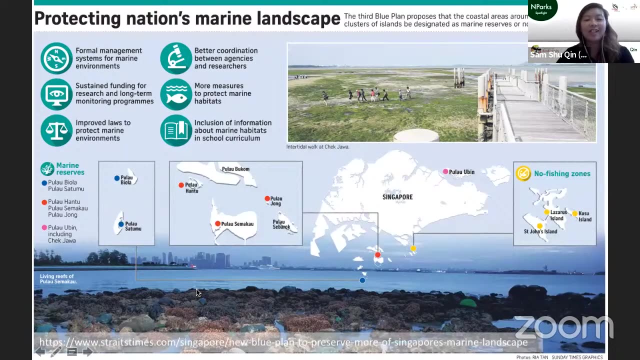 more integrated coastal management policies, and this led to the formation of friends of marine park community. and here we have the latest blue plan, the 2018 blue plan, and the new blue plan is a 2018 blue plan, so we can read more about it here at this link. okay, so in a nutshell, the latest blue. 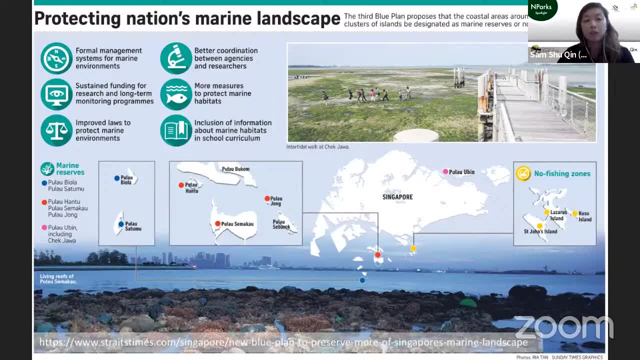 plan document proposed six recommendations to conserve the coastal and marine ecosystem, so we have six recommendations. so over here we have formal management, management of systems of marine environment, sustained funding for research programs, improved laws to protect the marine environment to have better coordination between agencies and researchers, more measures to protect marine habitats and to also include information about marine life. 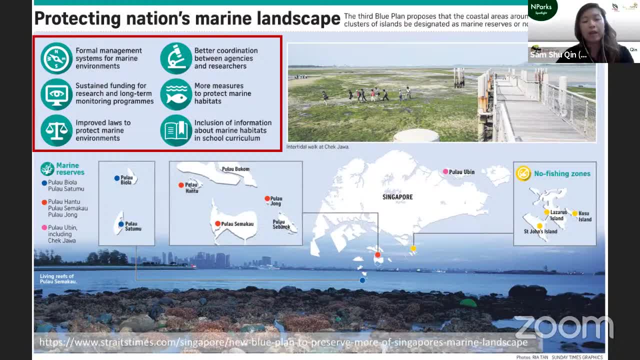 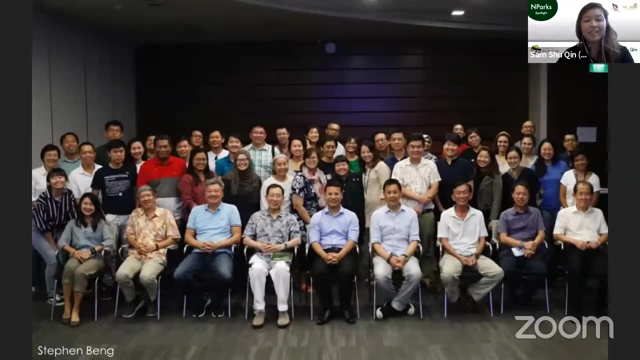 marine habitats, informal education. so with that, the blue can also identify more areas for protection. and we've had, with the formation of friends of marine park, a platform where different stakeholders can work together. we also hope to contribute to these efforts. so here this is my big family of friends of marine park community. okay, so the friends of marine park it brings. 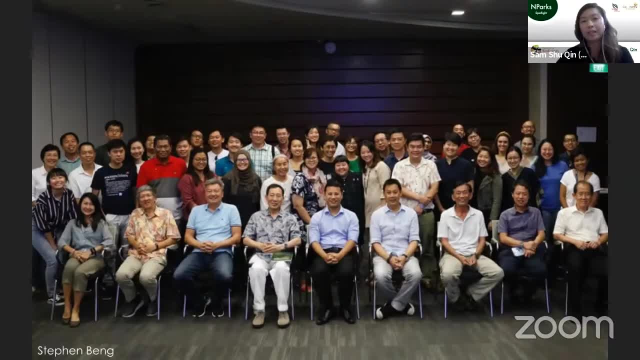 together people from all walks of life, from different expertise. we have boaters, divers, scientists, fishermen, kayakers, educators, amongst many- to pursue the common goal of managing the marine park as a place for all, for the community, by the community here and this network. it also encourages members to collaborate, talk to each other for the long-term survival. 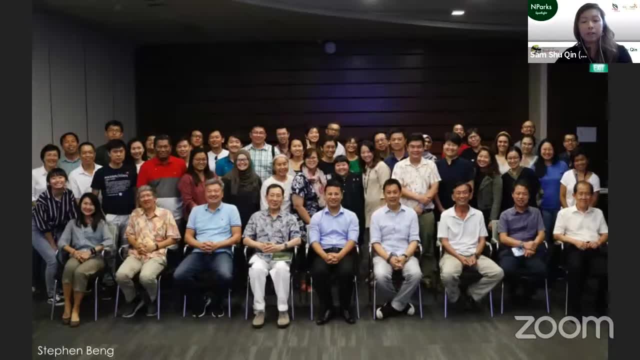 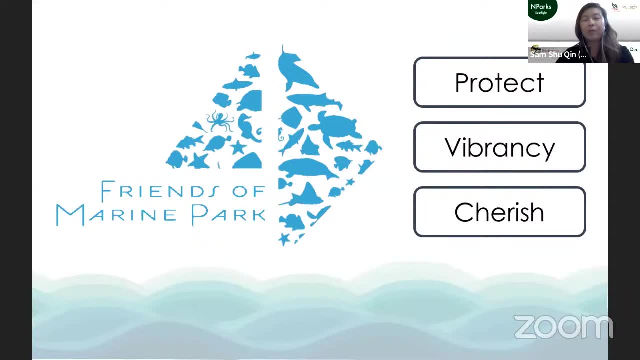 of life in our seas, and also to discuss and develop ground-out initiatives and guidelines to boost marine conservation efforts. So the communities always keep three main thrusts in our mind: protect our islands, to inject vibrancy to the marine park and to also cherish our natural and cultural heritage so that we can pass them down to our future generation. 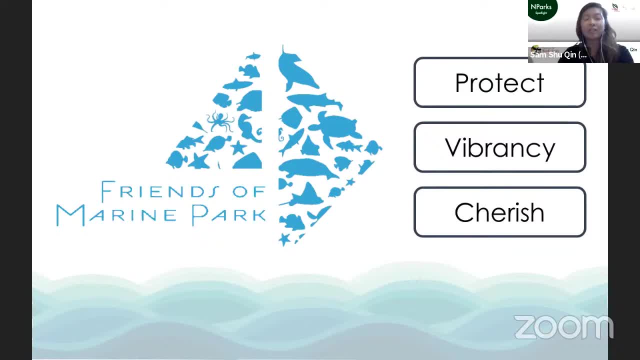 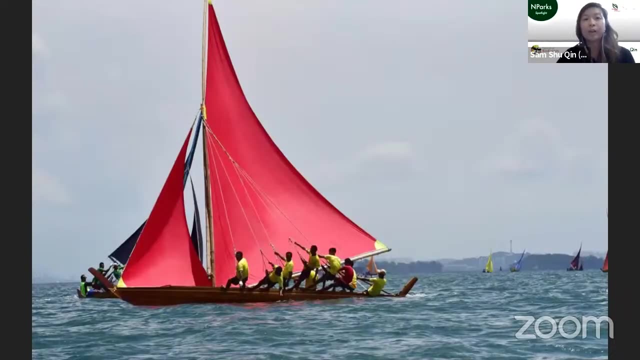 So you can see the cities. islands are also illustrated through the two triangles. So we have the small and big cities, islands reflected here, and the shape also resembles the sails of the colic boats which once raced around our southern islands. So we also work in five different domains. 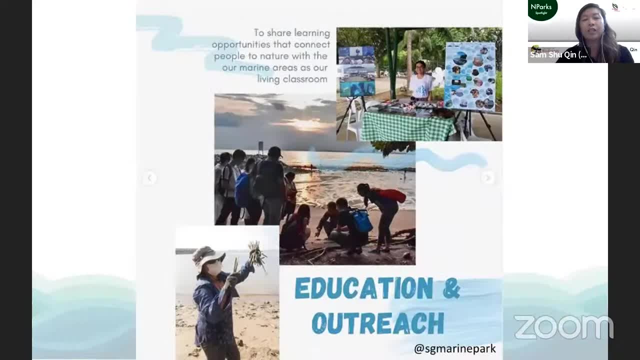 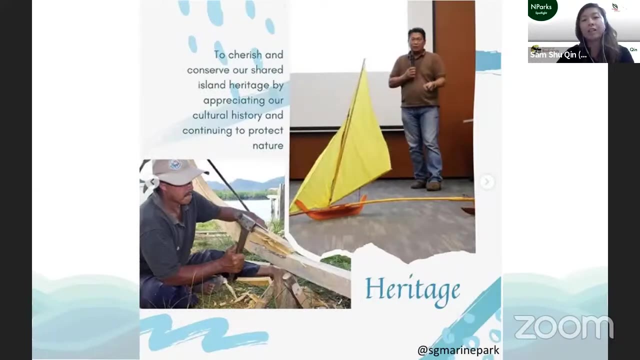 We have education and outreach- So these are the main goals- to share learning opportunities that connect people to nature, with the marine areas as our living classroom. So we have the heritage team to cherish and conserve our shared highland heritage by appreciating our cultural history, and also continue to protect nature so that 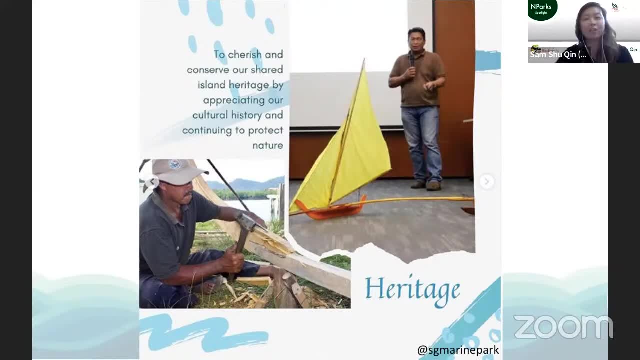 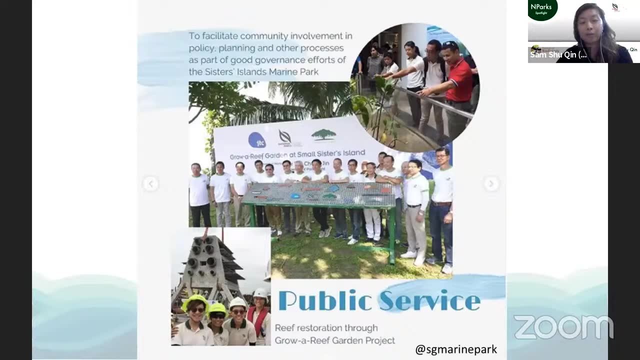 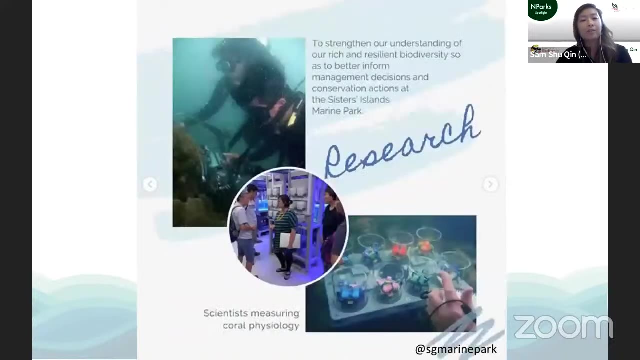 these stories will keep going on and pass down to the future generation. Of course, public service is very, very important to help to facilitate community involvement in policy planning and processes. as part of good government effort of the Seaside Island Marine Park, You have the researchers to help strengthen our understanding of our rich and resilient 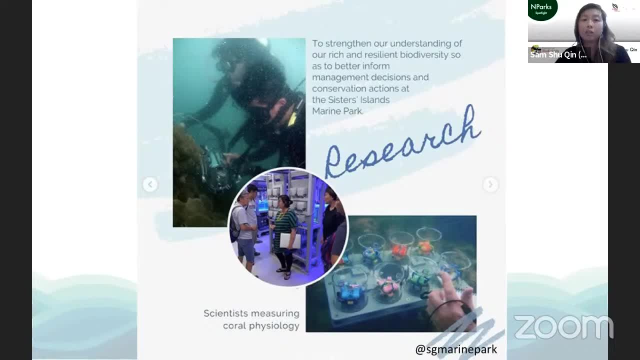 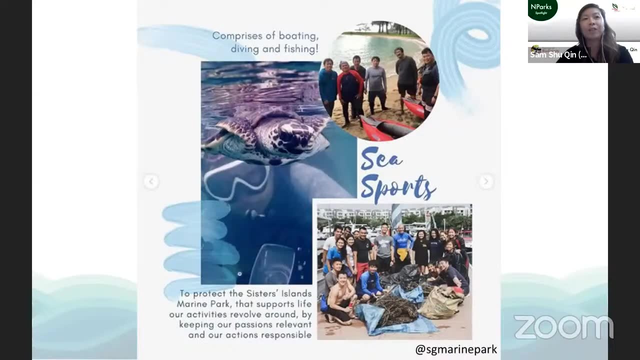 biodiversity, to better inform management decisions and conservation at the Seaside Island Marine Park. Lastly, you have sea sports. So sea sports are made up of different recreational users of the sea. You have the boaters, you have the anglers, you have the divers and kayakers. 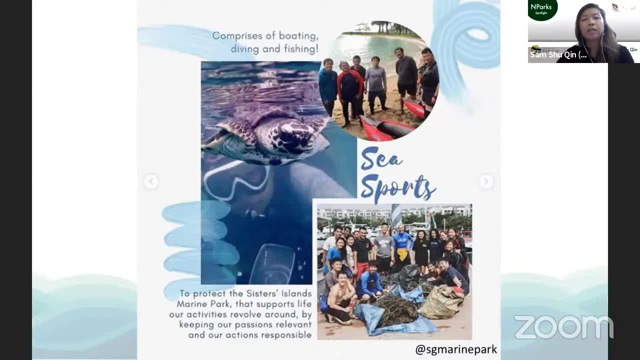 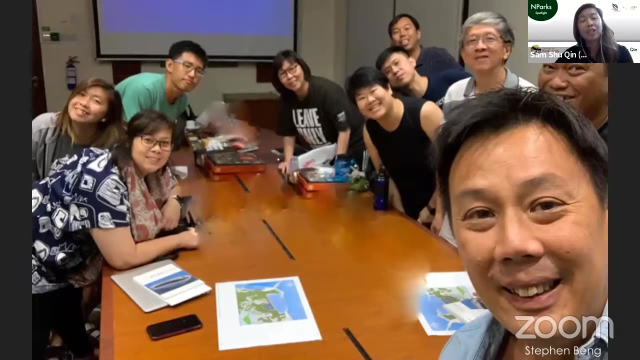 Okay, so you also want to protect Seaside Island Marine Park by keeping our passions relevant and actions responsible, and because of this, if you have a clean and healthy sea, you actually get to enjoy your sports even more. So for me, I float mainly between sea sports and research team. 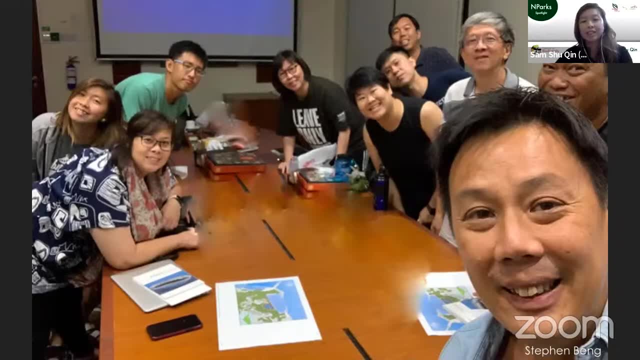 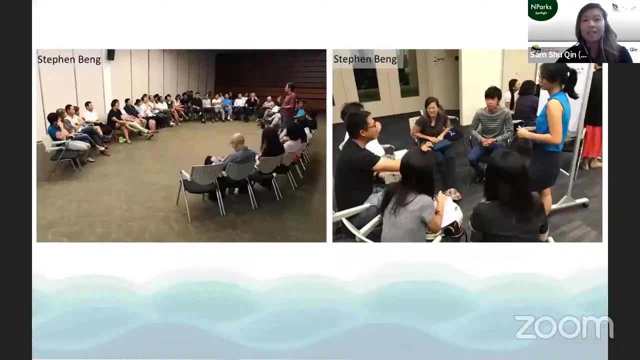 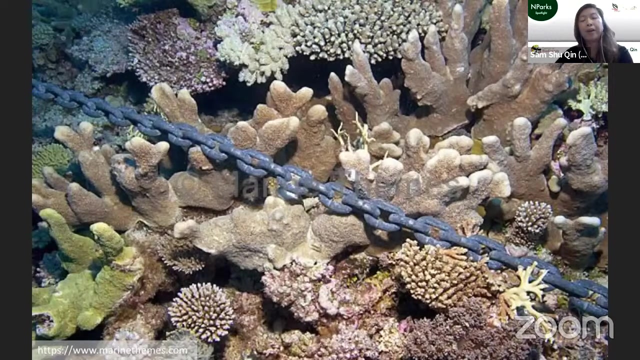 to provide my input based on my experiences in these two areas. So, as a coordinator, we help to manage multiple stakeholders activities and also facilitate discussion during the meetings. So here are also some issues that we have tackled as a community. Okay, so this is a picture of how an anchor chain can actually break and abrade corals. 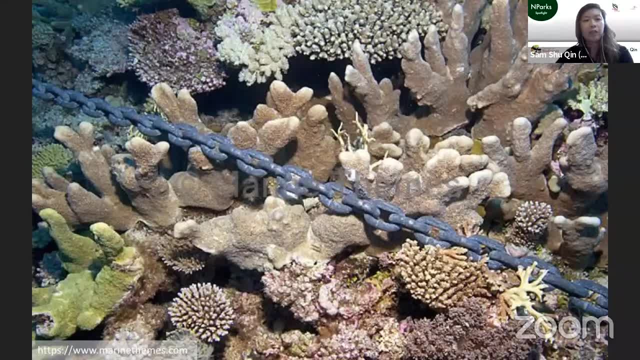 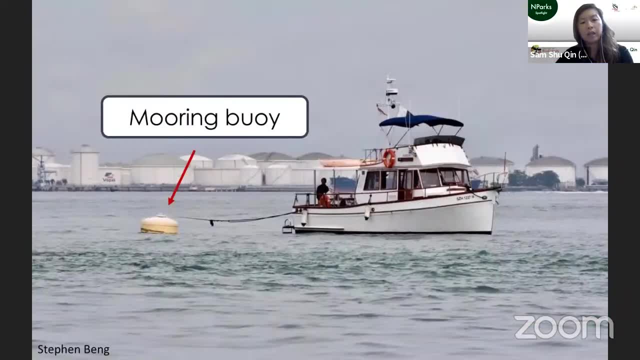 if they happen to land on coral reef and if it's not managed properly these anchors, they can also damage huge corals like this. So to encourage boaters and divers to visit the island but at the same time ensuring minimal damage to the coral reefs around the Seaside Island Marine. 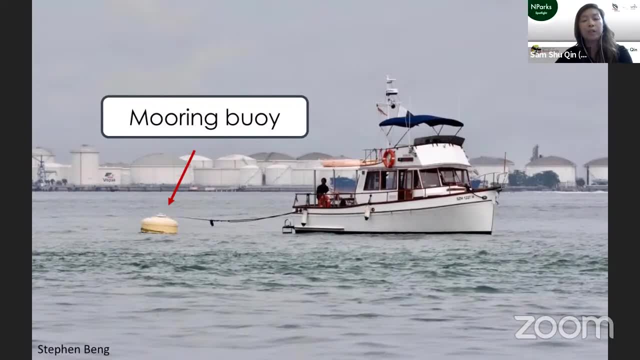 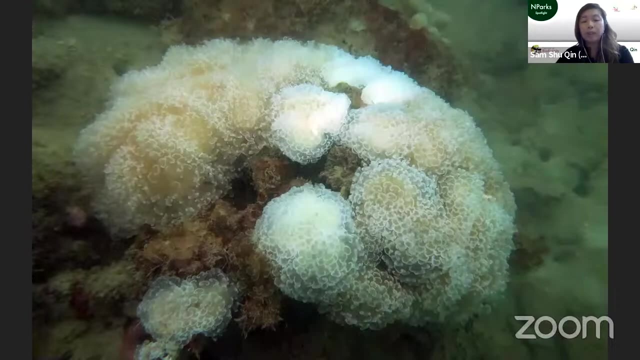 Park. the community proposed mooring buoys to be installed around big and small Seaside Islands to facilitate proper docking for these vessels, And now we have six of them around Seaside Island. So, also being in a community, it helps to amplify your voices and efforts. 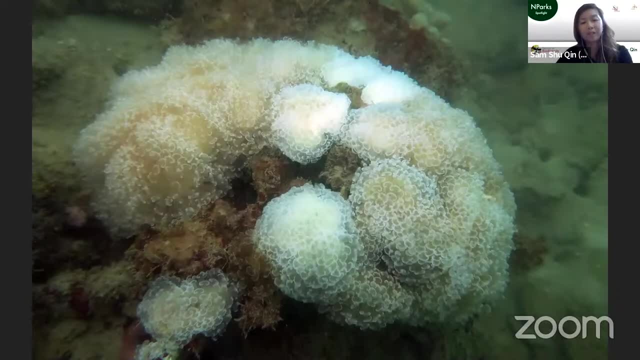 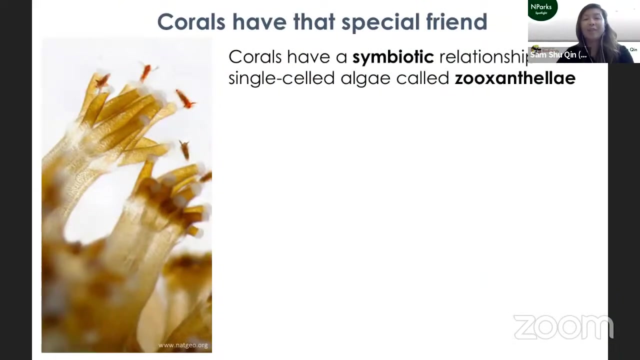 So, for instance, in June, during the circuit breaker period and during this pandemic, marine scientists we noted that there are some coral that were bleaching. Okay, so how does it happen? So, corals like you and me, we have a special friend right. so they have a symbiotic relationship with this single cell algae called zooxanthellae. 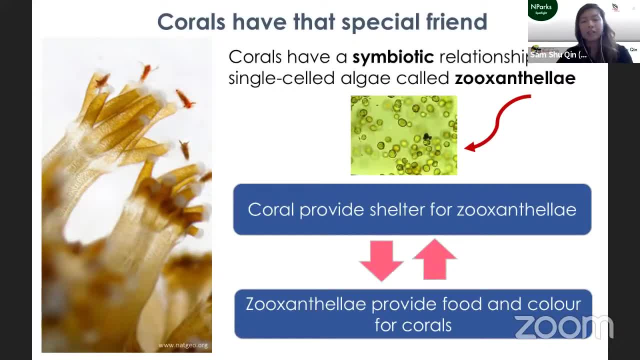 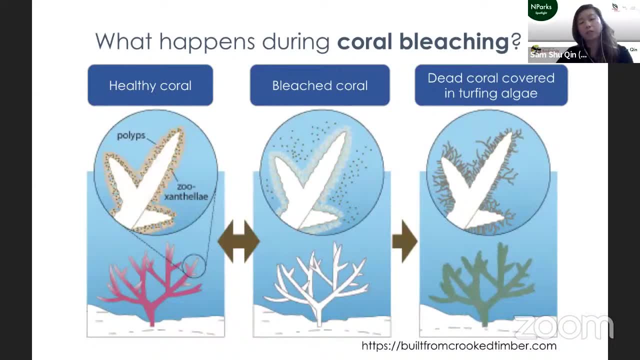 The corals host the zooxanthellae and in return the zooxanthellae provide food and color for the corals. So without the algae, the corals is deprived of its major source of nutrients. It then turns white whoops, it turns white or become pale. It can get sick easily also. 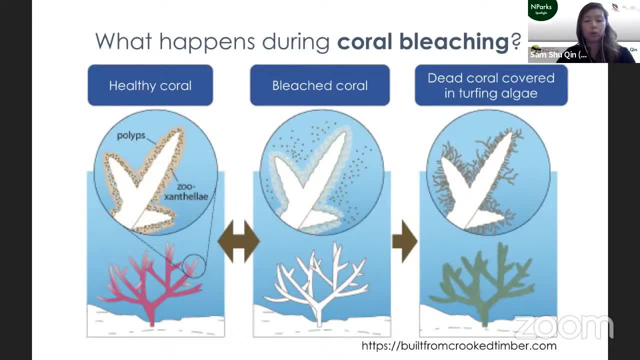 However, if the environmental conditions return back to normal or if the stresses are removed, these corals, they can recover back to their original state. okay, If not, if you see fairy things going on on the coral, it's probably that the corals are already covered in turfing algae. 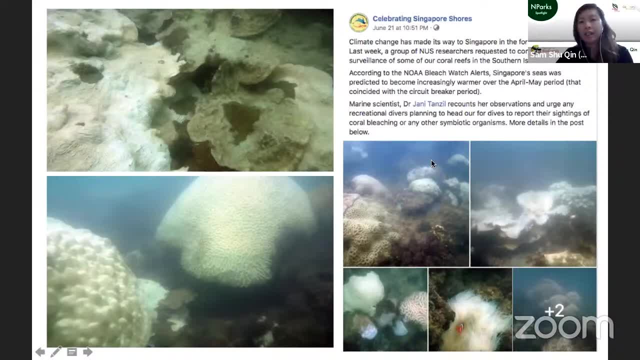 And through this coral bleaching events we can get a lot of data. so to help understand the extent of coral bleaching and also to find out the winners and losers of this recent episode, Marine scientists urged divers to report their sightings of coral bleaching or also on any other form of symbiotic organisms. 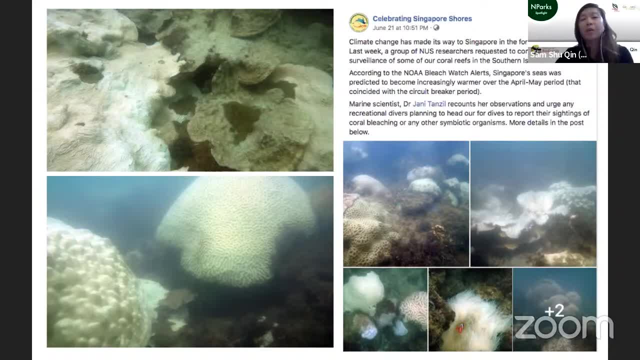 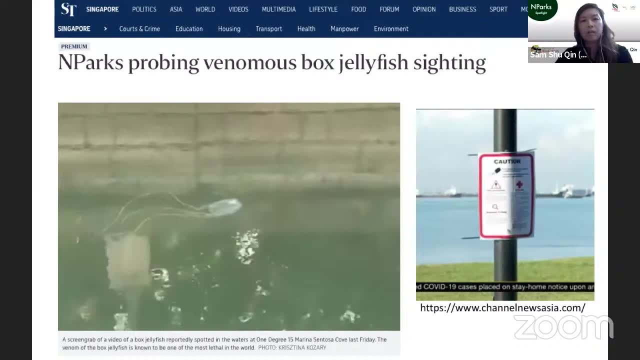 With friends of the Marine Park community. we also helped to share on social media and various platforms to amplify the message. Another recent incident is the boss jelly sightings at the marina by the Marine stewards. So because the community is in direct contact with the relevant agencies, the response time is short. 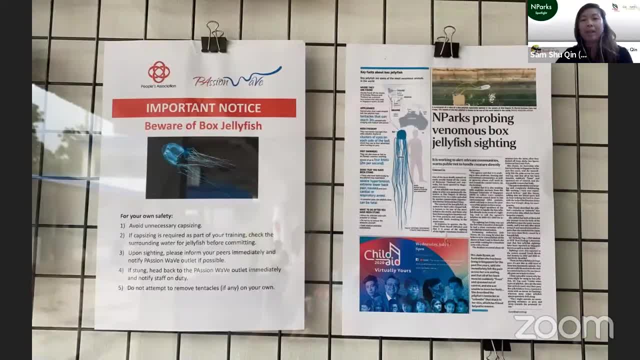 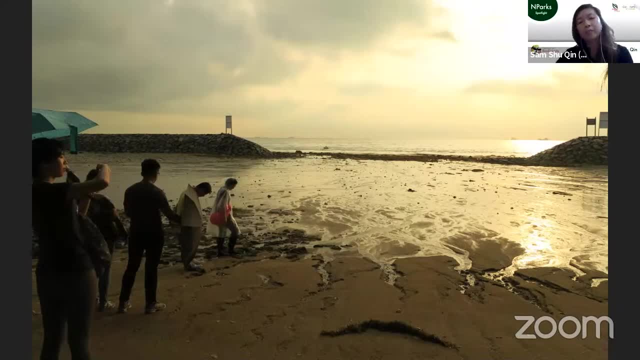 and therefore advisories and information can pass down to the public quickly. So the community also support the MPARC team with their efforts in public engagement and public outreach, such as bringing guides for intertidal walks at Citrus Island, And these are some of them sharing fun facts about the marine animals that they found during the walk. 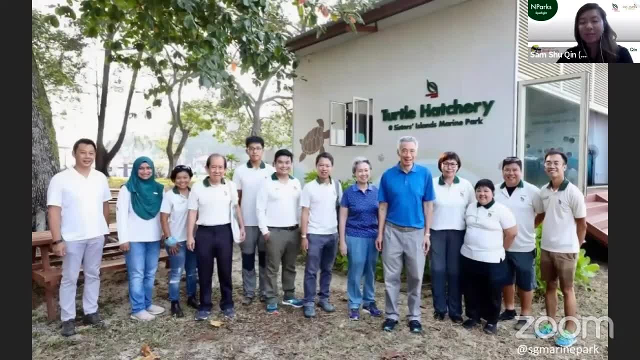 Thank you. There is also a turtle hatchery at the small Citrus Island, So this photo was taken when Prime Minister, Mr and Mrs Lee visited the Citrus Island Marine Park And, as a volunteer, I also have the opportunity to help release the turtle hatchlings. 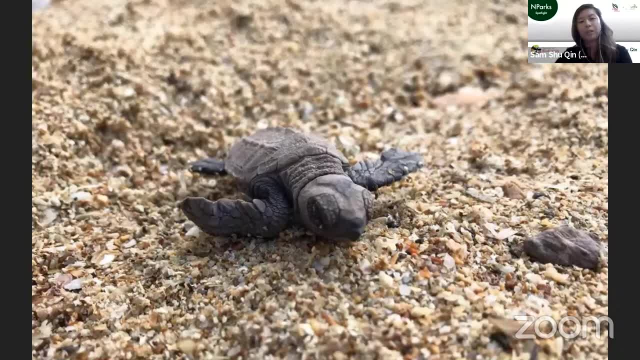 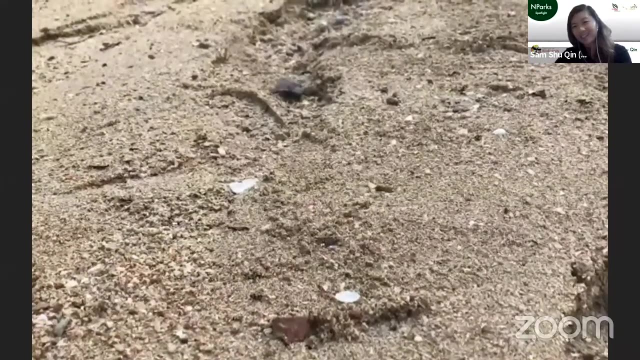 So the experience itself was magical. So before the turtles were released, we have to measure them, count them and see if they're in a good shape before we can let them go back to the sea, And then we place them near the shoreline and watch them walk slowly back to the sea. 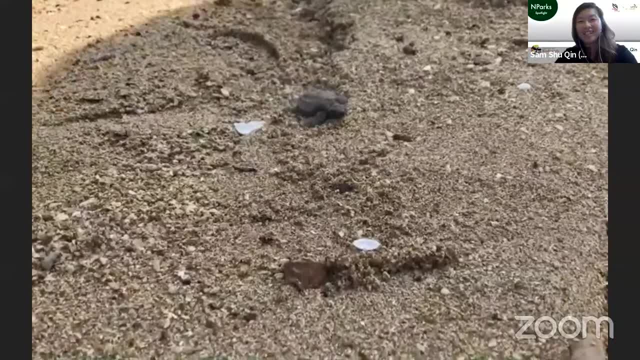 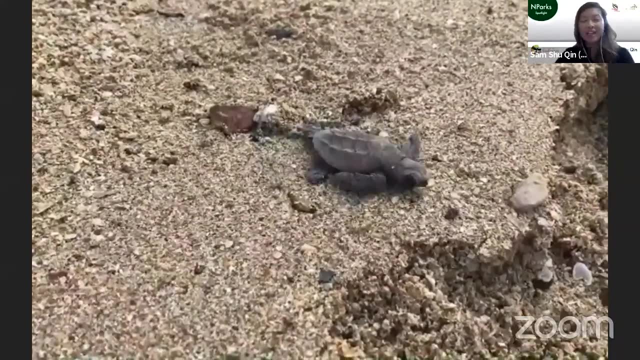 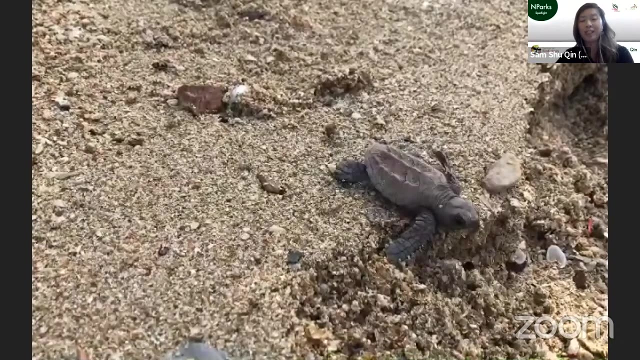 So cute, right? They're so tiny, So you can see a whole group of us carrying paths for them, making sure that they walk the right way. And there we go, we send them off to the sea, And sometimes you also go diving to look for treasures. 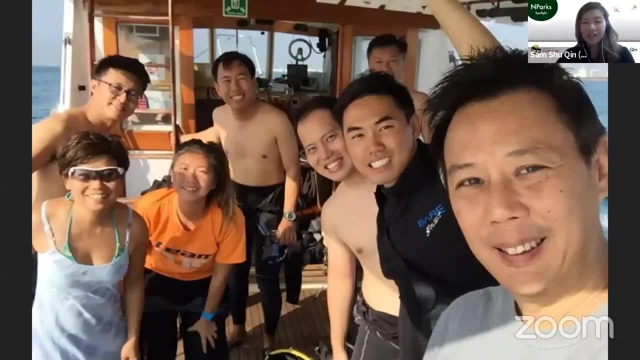 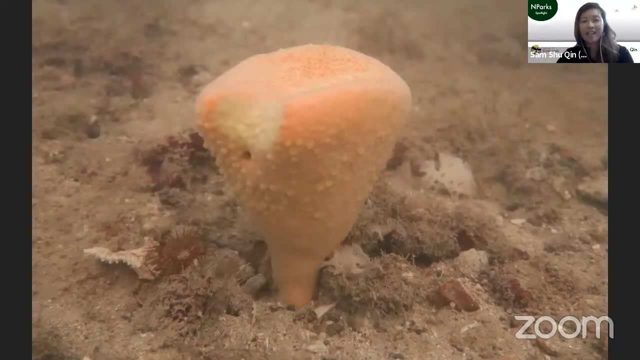 So, for instance, this is neppie. So neppie is a little Neptune's club sponge, And this species is thought to be locally extinct. So now they are in good hands, So yay. So there was also this dive where we chanced across a boo-boo trap. 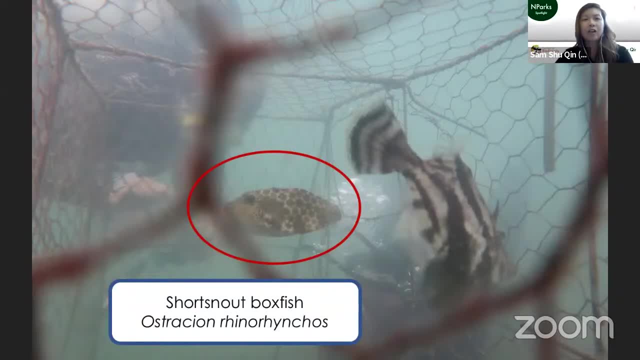 where there's some fish inside. So after taking a closer look we found that this boxfish. it looks kind of special. So we took photos and we sent a photo to our fish experts at the museum And we were pleasantly surprised that it was a rare find. 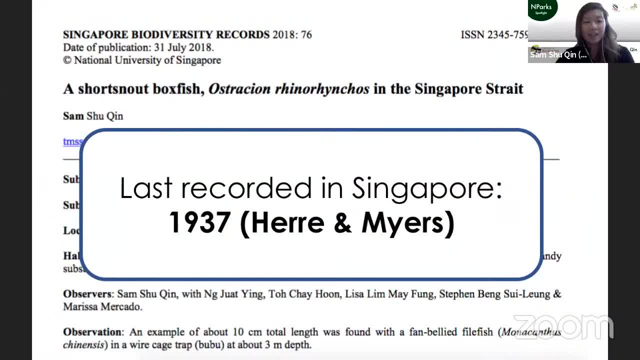 So this fish, the short snout boxfish, was actually last recorded back in Singapore in 1937. So this is also counted as a rediscovery of a newish species. So I submitted it to the museum and this is actually published. 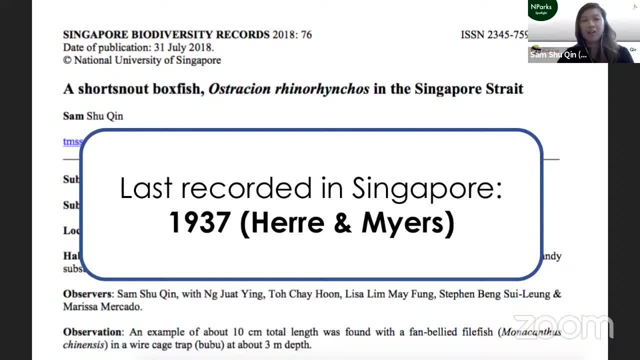 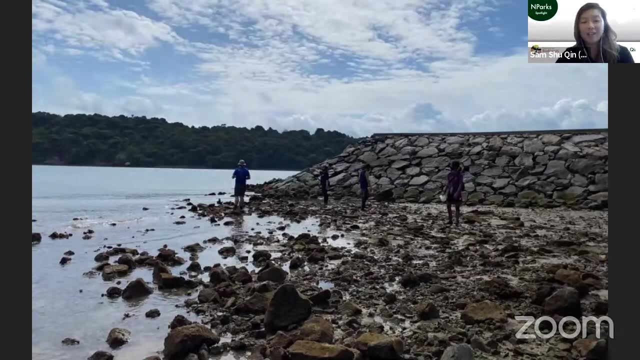 So we also encourage divers or even anyone. if you chance to cross weird-looking species, take pictures and send to the researchers. Maybe you'll find something new in Singapore, Okay. So the community also likes to explore, So there is also a community space at St John's Island. 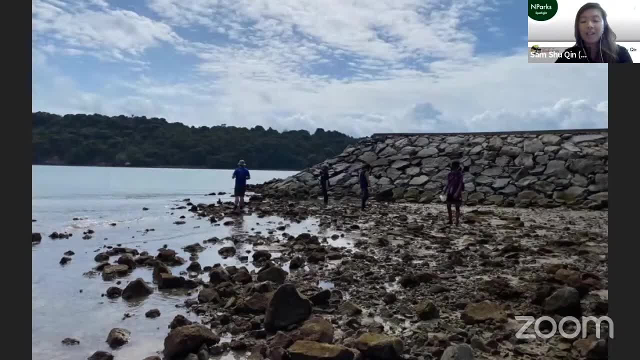 that we are hoping to use for future public engagement programmes. So the team headed there at low tide for a recce trip to see what kind of animals we can find at that area. And these are some of the gems that we find: We have sea cucumber, a lot of sea stars, sea grass. 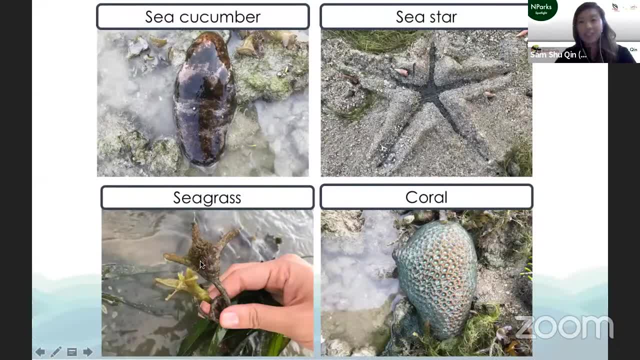 And this is interesting because they are actually flowering, So it's actually a good sign And we have a lot of corals right there. And, of course, how can we miss this marine debris? Look at those bottles, I see already my hands are really very itchy. 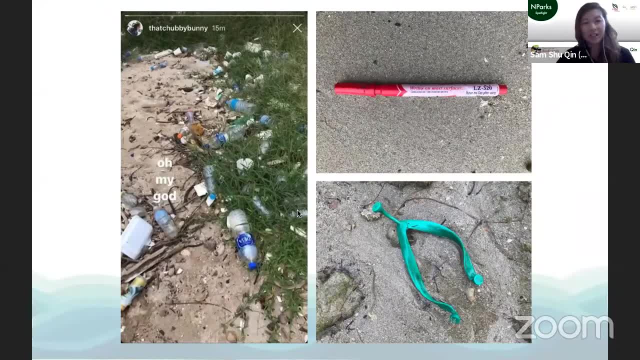 I want to pick them all out, Okay. So what happened was because of all this, during this year's National Day, a group of us went to the beach to clean up the area, Okay, And this was organised by the education team of Friends of Marine Park. 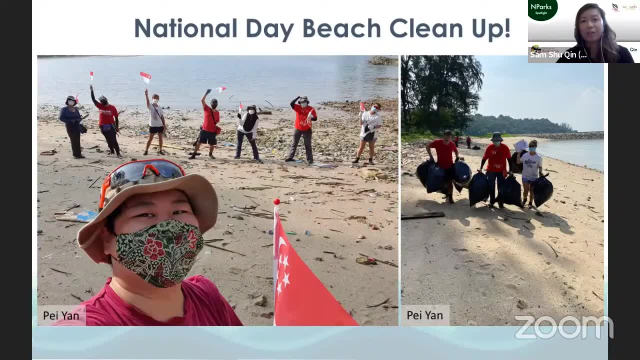 And within a short one hour we picked up a total of 26 bags of trash And they weighed almost 130 kg. So all this trash are packed up And then it will be packed up, packed nicely, and disposed back on land properly. 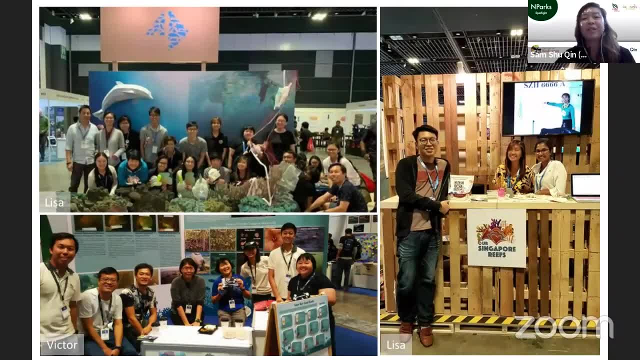 Okay, So the Friends of Marine Park community. we also have events like Festival of Biodiversity and ADEX, the Asia Dive Expo, to share our experiences and also to raise awareness on local marine conservation efforts. So this year ADEX went virtual. 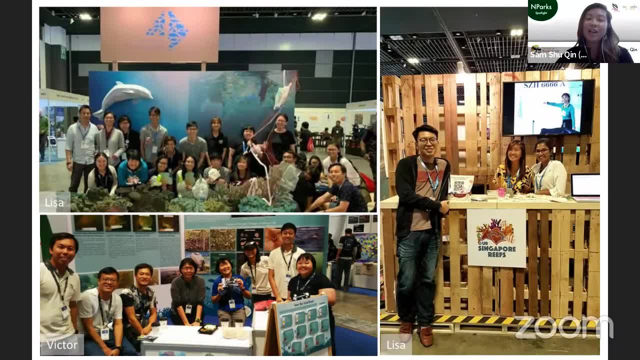 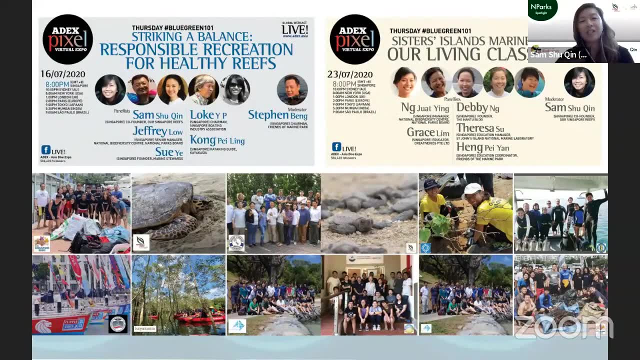 And we also took the opportunity to arrow- I mean showcase- our people and our work. Okay, So, thanks to the ADEX team, we managed to run a series of four sessions to introduce our teams. So we have the sea sports team talking about how you can actually have a balance. 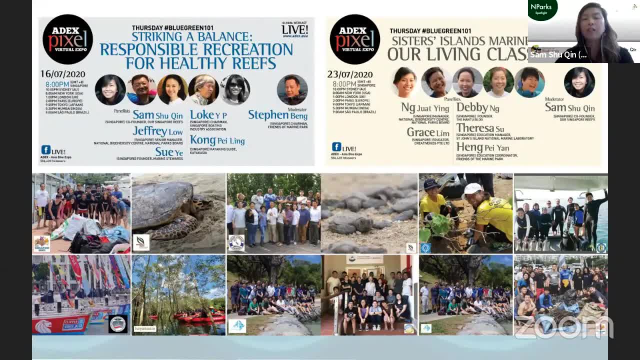 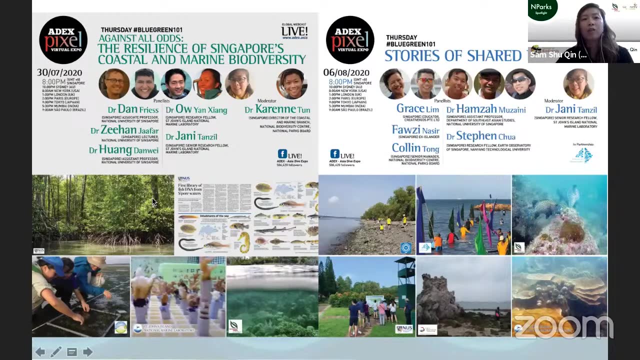 between having a responsible recreation and healthy reef to keep them healthy. And also we have the educators talking about how to transform Sisters Island Marine Park into our living classroom. You have the scientists that come on board to talk about how resilient our coastal and marine biodiversity are. 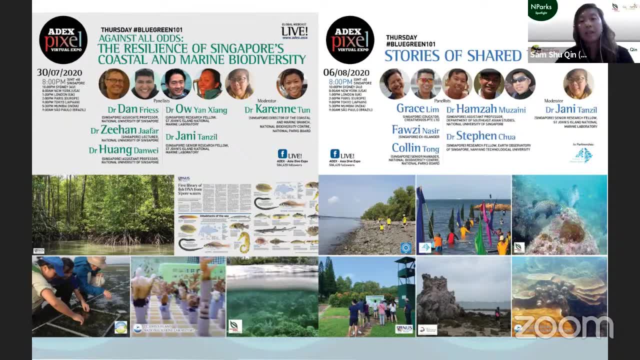 even though they're under a lot of stress from coastal development and habitat loss. And lastly, all those stories from the past. It's really a time capsule where our friends from the Culture and Heritage team brought us back all the way back to life on the island. 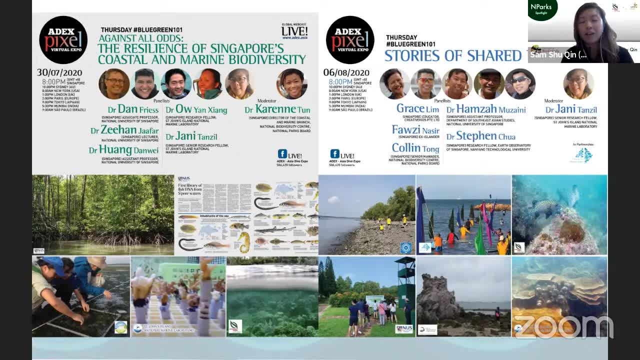 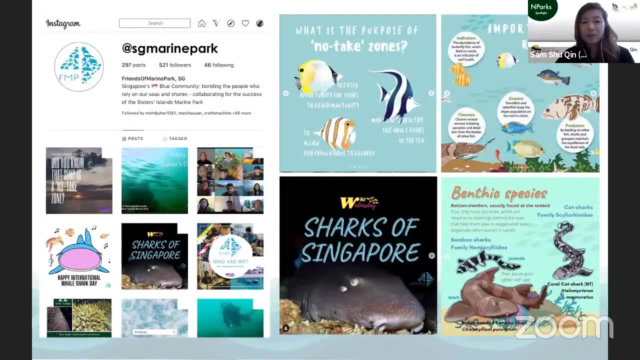 And also how our natural heritage- the coral reef and the rock there- are also very important, And also to keep online engagement going. the younger ones also took over our Instagram account, So do follow us to find out more about our marine environment and the animals living within. 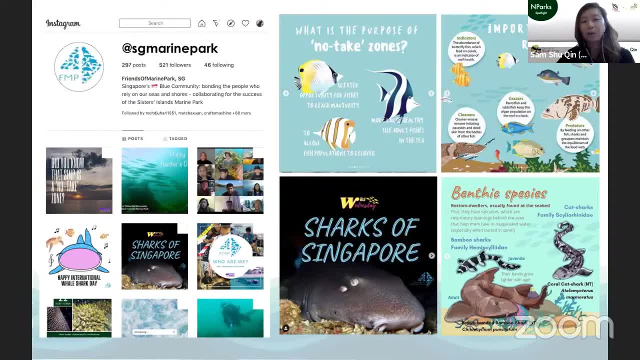 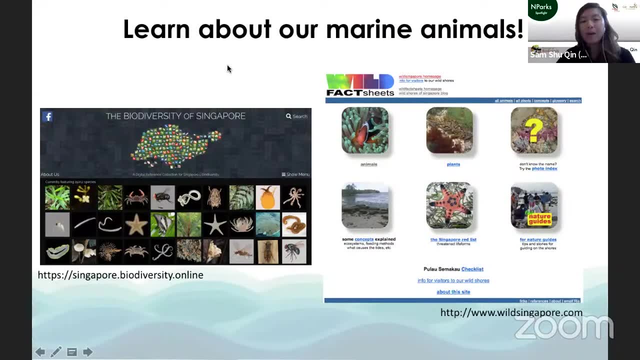 and also to keep updated on what the marine community is doing, So also to learn more about what we have in Singapore. you can also check out these resources. So you have this biodiversity of Singapore, and this is from the museum, the Continental Museum. 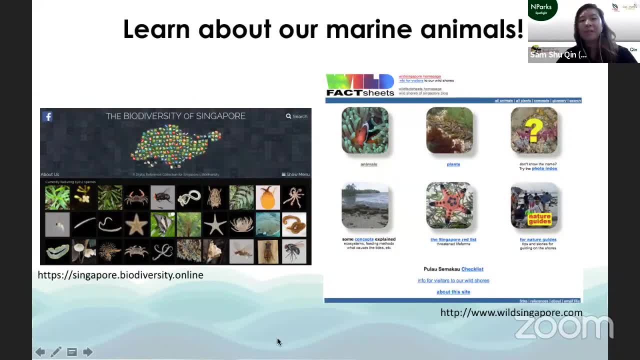 And you have wild fact sheets from wild Singapore. So this is where, when I'm not sure what I'm looking at, or if I want to find out some of the animals what they actually are. these are some of the database that I actually 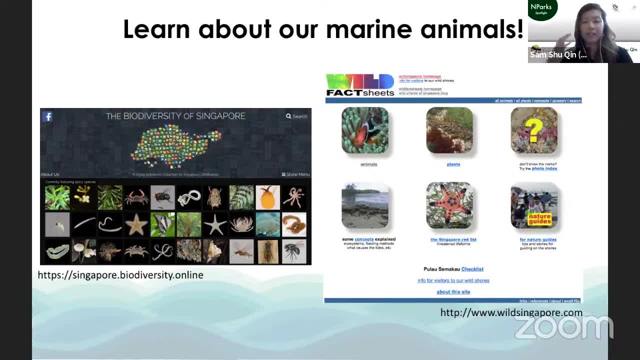 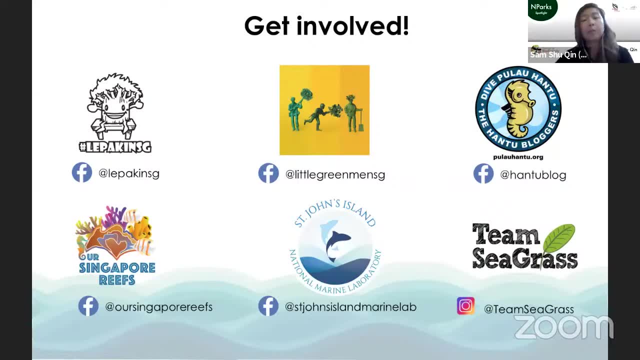 could find and discover, And also I want to encourage you to get involved in marine conservation. So here are some groups that we can follow. We have Lepa in SG and Little Green Man. they are run by amazing youth. You can find listings of environmental related events. 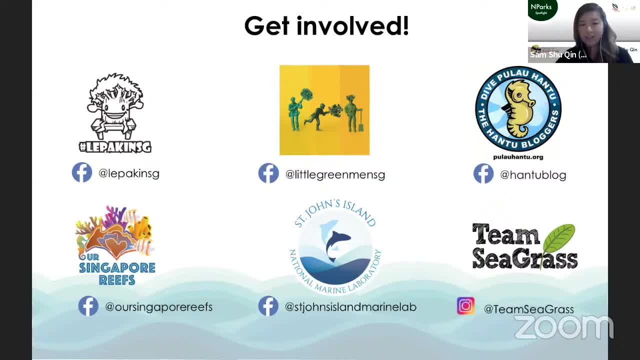 and activities at Lepa in SG, Little Green Man. they organise coastal clean-up So you can join them if you're interested And to explore Singapore's reef by diving. you can reach out to Hantu Block and our Singapore Reefs. 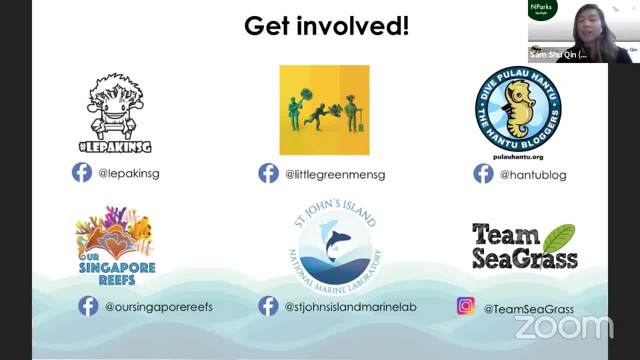 If you want to know more about marine science, you can follow St John Island's Marine Laboratory, And also if you are interested in going out to the field and getting your hands dirty and also learning a bit of science, you can contact Team Seagrass. 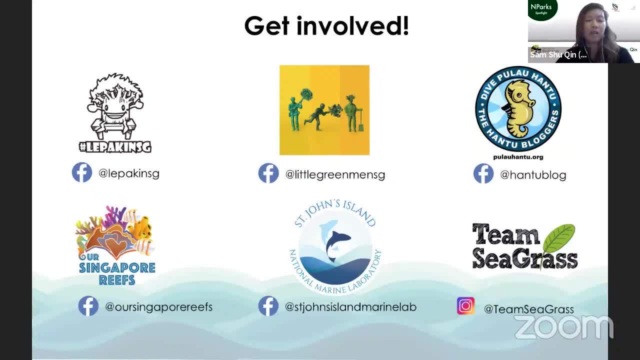 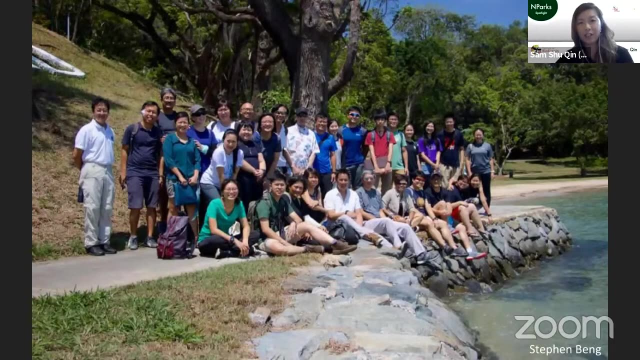 for season science opportunities. So there are still so many groups out there doing such great jobs, So please do a little search on them also. You might be able to find what you like. So I must say, throughout my marine conservation journey, this family has been such a great push. 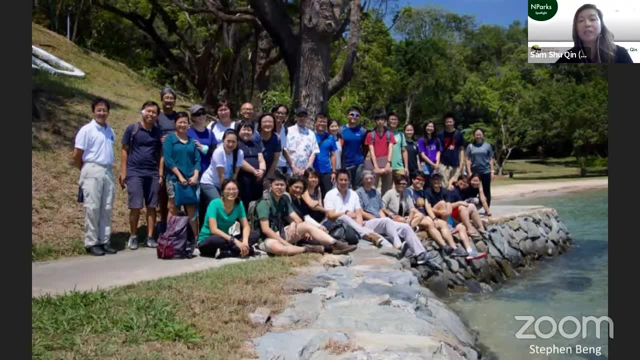 So the support from the marine community is very strong And it's really like the old kampong spirit. You share your ups and downs, they will cheer for your success and they are there when you hit a roadblock- And many of them here. 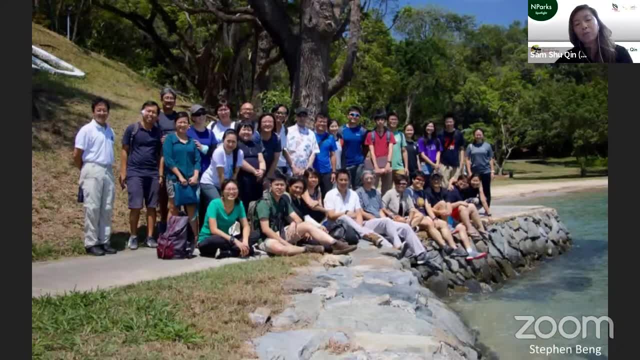 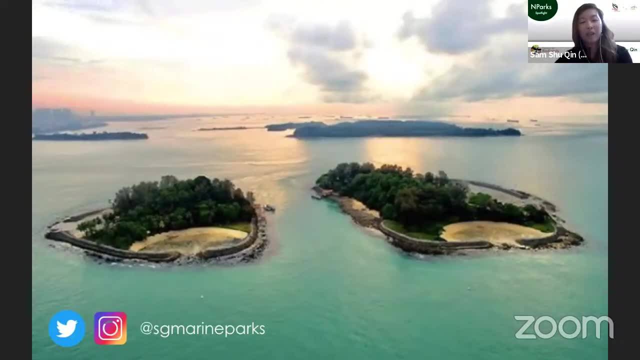 they inspire me to want to do more for the community and for the environment- And that really keeps me going- And, of course, to protect and conserve what we have- our natural heritage. the community also needs all of your help to do your part for the environment. 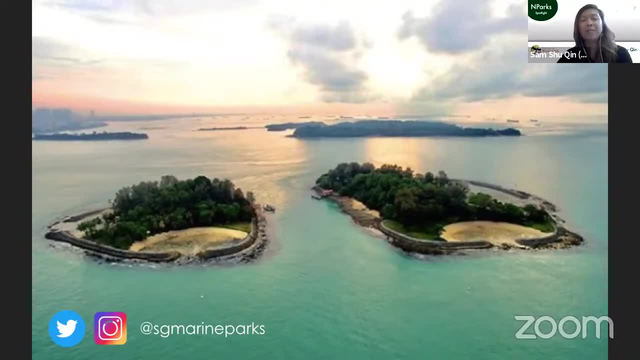 So it can be just as simple as being a little more conscious of your own action, because whatever this little thing that you do, it can set off a certain impact to the environment Or, you know, you can even go out there with your friends. 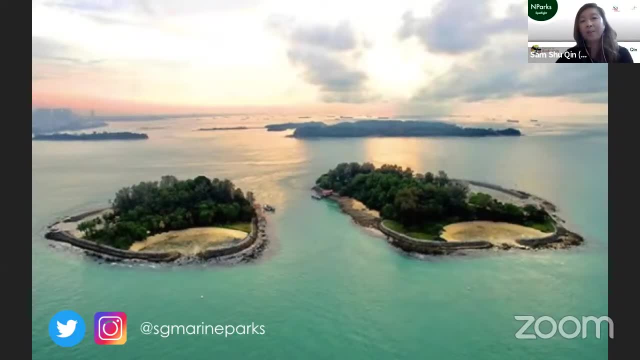 with your families to rediscover our green and blue spaces. So we really need all of you to go there and see what we really have, because if you know what we have, then you know how to protect them and cherish them. Okay, So with this, 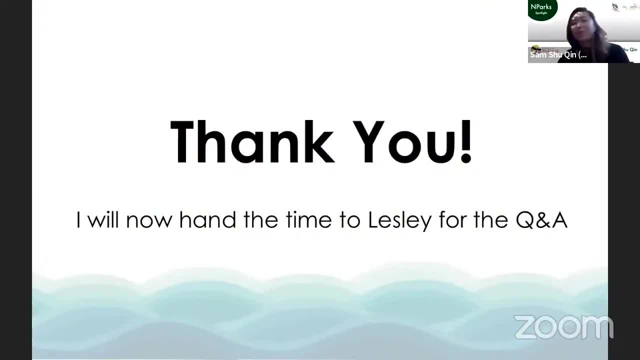 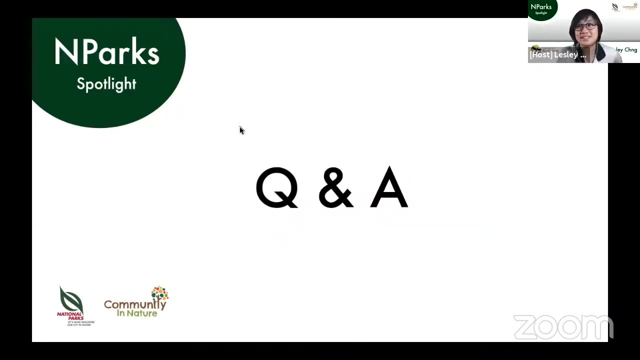 I end my sharing and I will now hand the time over to Lesley for Q&A. Thank you. Thank you, Sam. Okay, let me just share my slides and we'll move on with the Q&A. Okay, So the first question for you, Sam. 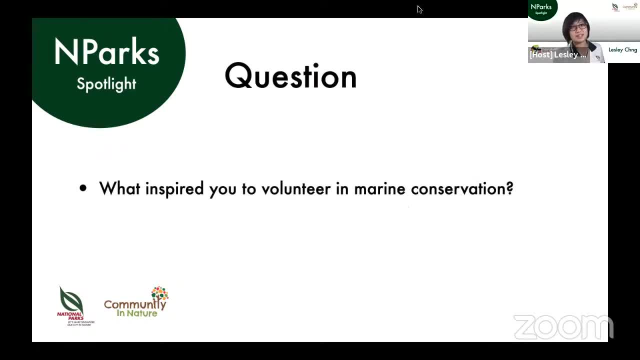 is what inspired you to volunteer in marine conservation, So this is actually a good question. So from young, I was very attracted to the sea And also, as a user of the sea, I wanted to give back, So spending a lot of time underwater. 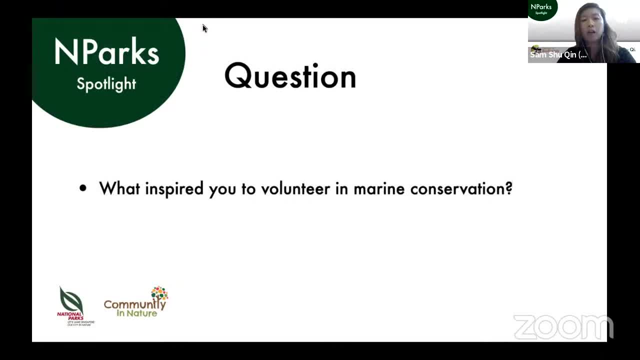 for work and leisure made me realize that you know how coral reef and the marine animals within they are also precious and at the same time so fragile, And because we don't get to learn about all these marine animals and the state of the ocean. 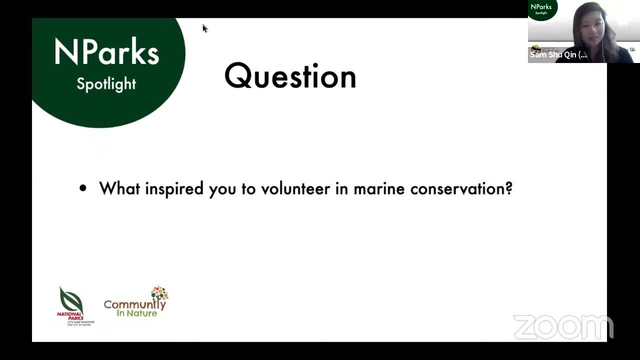 and environment in our formal school education. I want to reach out to the public, especially the younger ones, with what I've learned from years doing research and through this engagement with the public I also hope that you know people can go out to the sea. 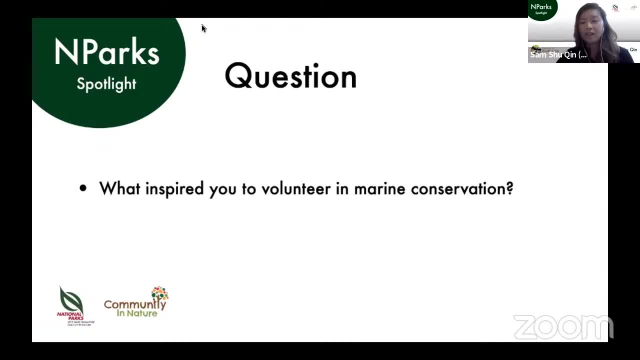 go out to the coastal habitat more often so that they can be more aware of the rich biodiversity that we have, and to realize that, you know, at the end of the day, the sea and us, we are all interconnected in that sense. So it's very nice to hear. 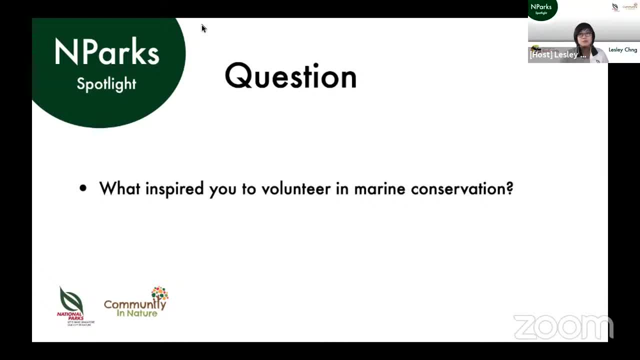 that you were inspired to give back and you make use of your own knowledge, your own background, to help bridge the gap between knowledge about the sea and the community. Okay, the next question: What is your favorite marine animal? Wow, this is a tough question. 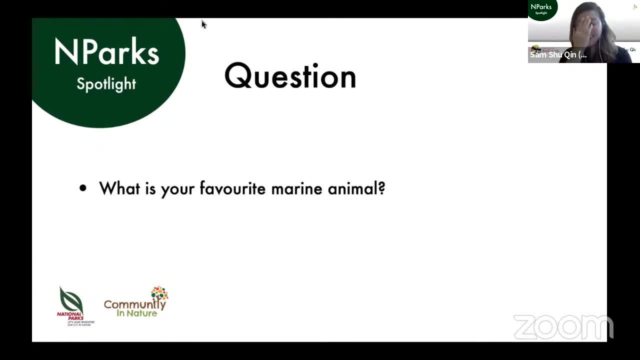 I have so many favorites I cannot answer Okay. Actually, I really like sharks, So my favorite favorite favorite is great white shark, And I had the opportunity to go to South Africa to do an internship with great white shark during my final year. 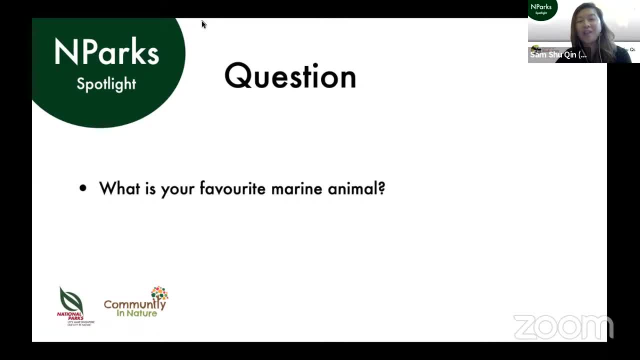 as a final student. So that is how and why I really wanted to do marine biologist. So after you come back to Singapore, it's like, ah, there's no great white sharks here, And the sharks here are like small. So okay, everything is important. 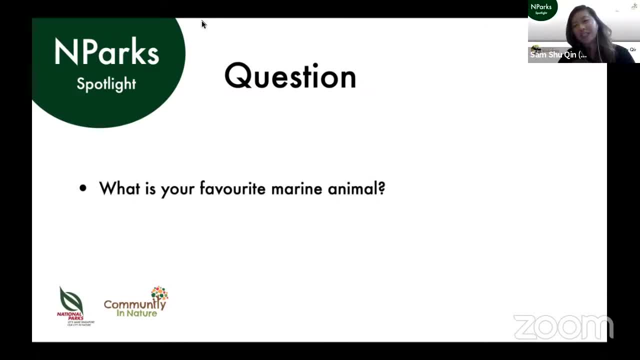 But currently the top one is still great white shark, But I have still I have a lot of favorites, So I'm still a shark person. Okay, So even though we don't have great white sharks here, we do have other types of sharks, right? 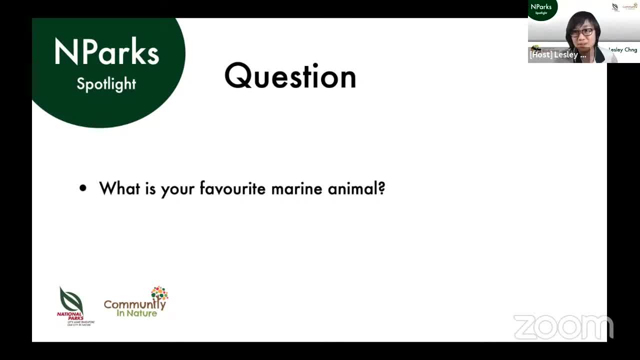 So what are some of the? what sharks can we find in Singapore? Oh, we have bamboo sharks, We have coral cat sharks, Yeah, And then we have a lot of reef sharks. So black tapes, we have them also, So they're all hiding. 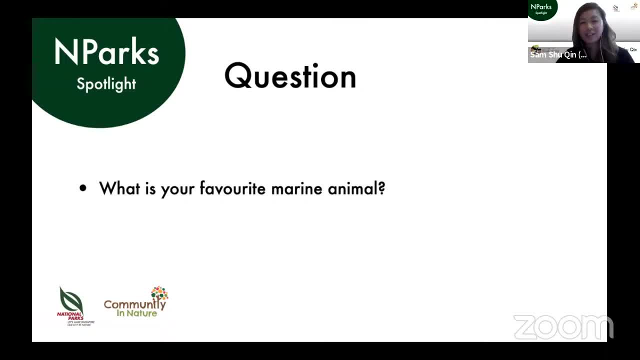 You need to have good eyes and patience to spot them and a lot of luck. So throughout my years of diving- I think four or five years- I only seen twice. Yeah, But there are also groups working on sharks, So let's say bamboo sharks. 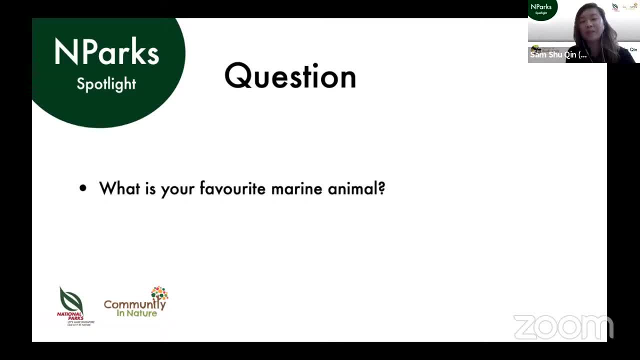 you have the team from James Cook University. They're actually looking for them. So if you happen to spot any shark, do feel free to take pictures and send it to them. Okay, So we do have a few species of sharks In Singapore, which Sam named. 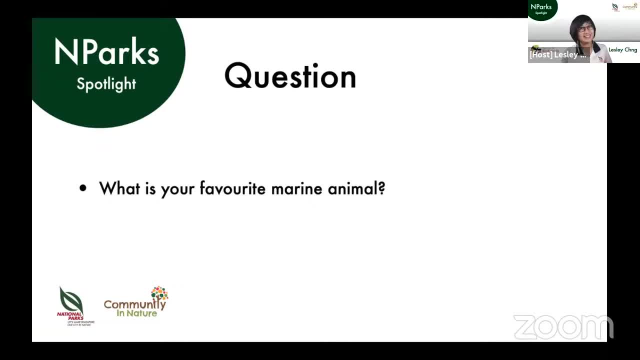 And even though it might be hard to see them, they are there and they are actually groups dedicated to studying some of these creatures. All right, The next question is: I'm new to marine life. What are some common species I might find along our shoreline in Singapore? 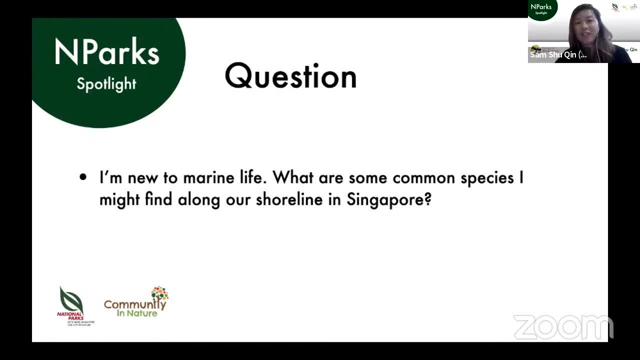 So this one, I'll encourage you to actually go out during low tide. So find the days with low tide, go out to shore that actually really accessible, like East Coast Park Pasir Ris, So just go there and have a little walk along the beach. 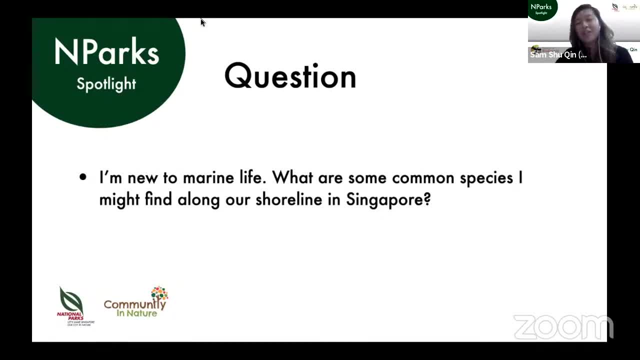 And you might find things like sea cucumbers. you find sea stars, And then you also see, if you're lucky, you can find some sea slugs which are really interesting. Okay, They can be really colourful, They can camouflage. 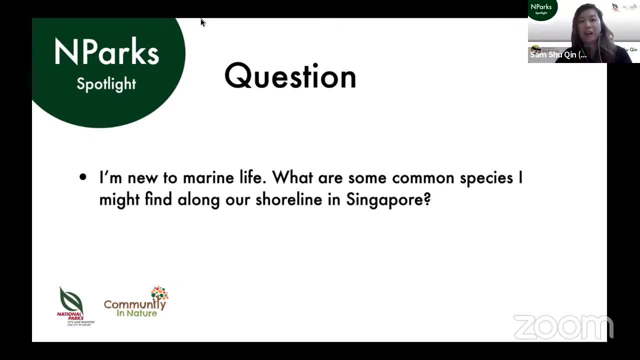 But do be careful also, because sometimes we have stone fish that can easily camouflage themselves and they look like rock. So if you want to take a walk there, so just be careful to wear covered shoes and look where you step. So corals are also there. 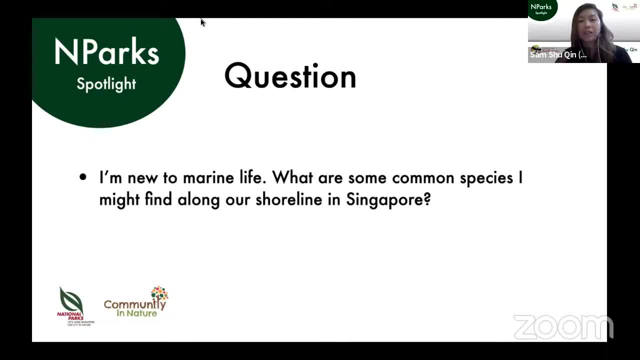 So different habitats feature different types of animals, So do take some time to go to different areas to explore in that sense. So if you want to find out more, I think NPAS is also doing guided walks at St John's Island, So there are also groups out there conducting nature walks. 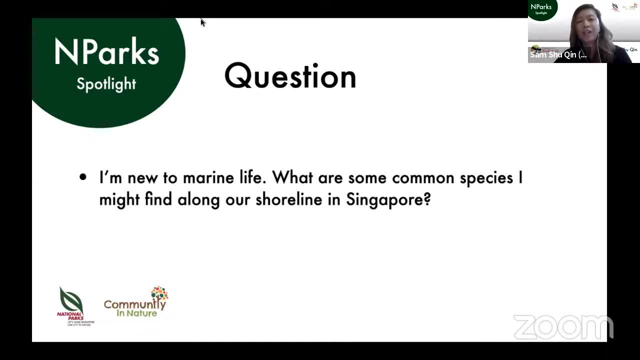 So do feel free to reach out to them also so they can actually share more, And they are actually very good with spotting these animals. Okay, So just along our shoreline, the intertidal area, you can find a variety of creatures like corals, sea cucumbers. 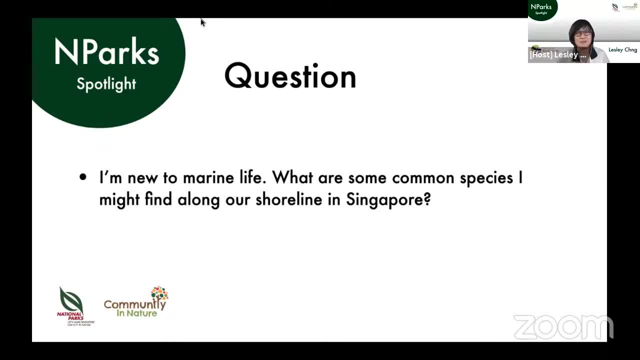 even sea slugs, And you don't have to travel too far from the shore to see them, And, as Sam mentioned, there are several groups that offer guided walks if you want to learn more about these creatures, And at NPARCS we also have an intertidal watch programme. 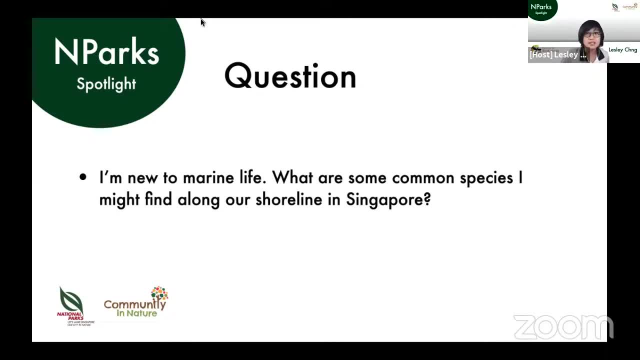 where you can be trained to identify and help document these creatures, And I think maybe later on we'll try and send you the link to that page if anyone is interested to find out more about this programme. So hope this answers the question Next. 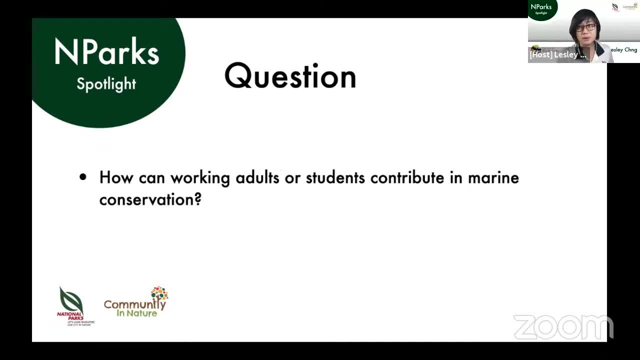 How can working adults or students contribute in marine conservation? So I really encourage working adults and students to get involved. So if you are really interested in marine conservation, so volunteer a little of your time or resources you know to organisations that can. 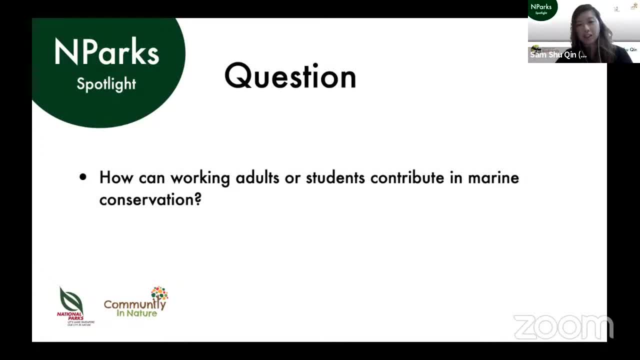 and all these resources can be really useful for some organisation. So for students, if you're interested in marine conservation, it's good to start volunteering or getting some internship with some of these groups here, So you can even start a project or campaign in your school. 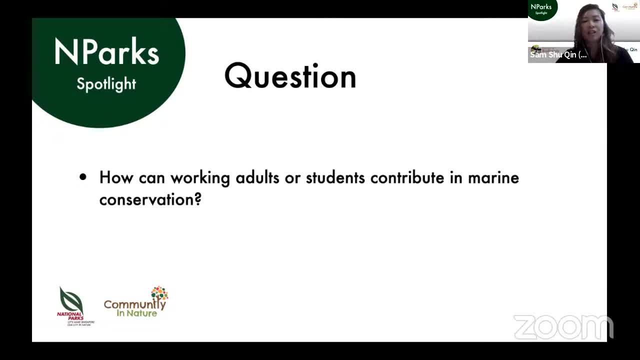 to get your friends interested in marine conservation or to know more about certain marine animals. So feel free to reach out to anyone in the marine community So I'm sure they'll be most happy to help you to do all these projects. to fact-check: 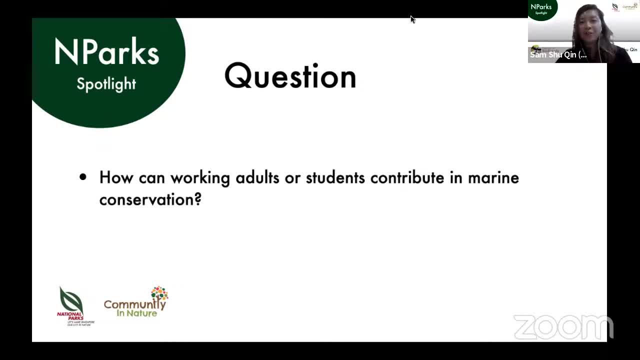 to come up with ideas. So, yeah, Do feel free to reach out to us. I think Sam shared a lot of resources earlier, a lot of groups that you can reach out to, and I'm sure they'll be more than happy if you approach them to volunteer. 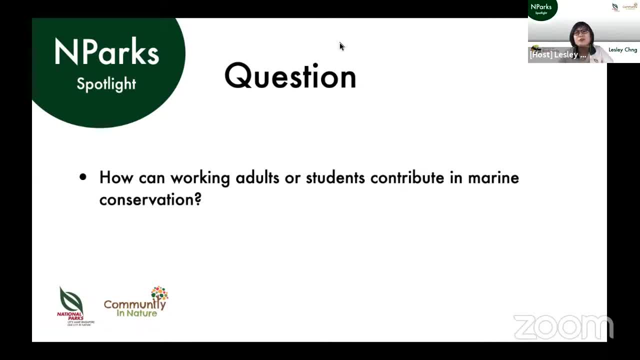 And you can start small, your own circle, your own school, your own family and friends. Okay, Next question: How does trash on the beach affect marine life? So this is a question I get a lot. So if you, especially during this season, 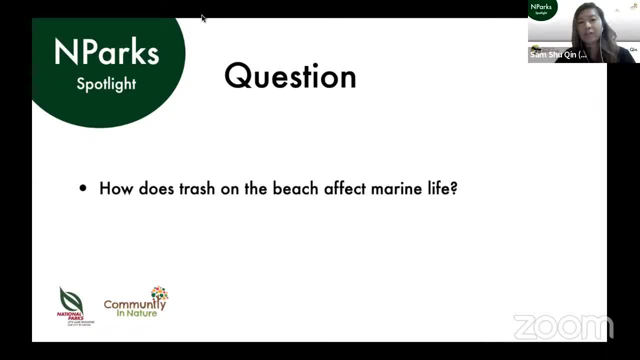 you know, you've seen a lot of news report on how East Coast Park has a lot of trash, right. So this trash on the beach, if they go to the sea, okay, so they might end up entangling some of the marine animals, right? 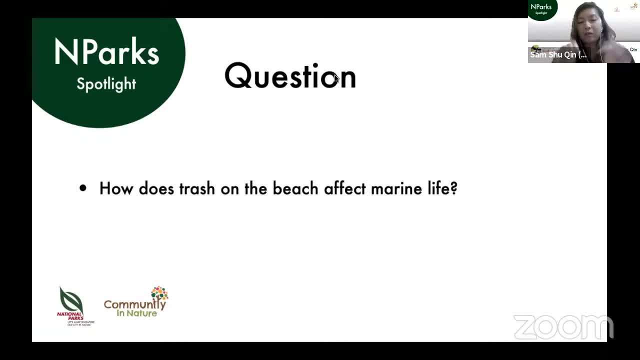 And then if they are small and they break out into tiny pieces, micro plastic or micro fragments, they might end up in some of the marine animals stomach, because they don't have good eyes like us. Okay, So they might mistaken them as food. 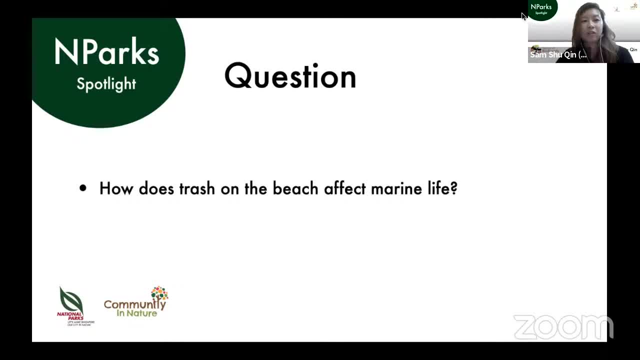 So bigger trash, like glass bottles, you know, you have your big cylinders, you have big containers, bicycles, all these things, if they end up in the water. so what happens is they can crush and destroy some of these coral reefs that are home to marine life. 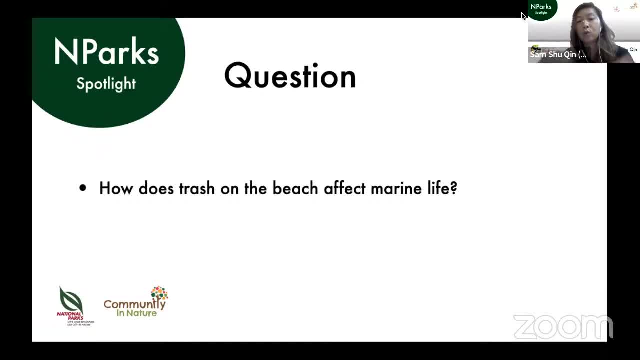 right. So in corals they actually take very long to grow, So for them to recover back it might take a long, long time And because their homes are destroyed, the marine life had to find some other place to stay. Okay. 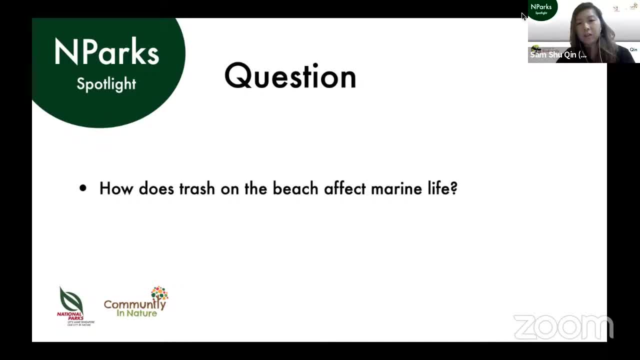 So the trash on the beach also, So some of them. we might find animals being trapped And okay, so trash, let's say like containers or like bottles. some of the animals can find their way inside and they might not able to get out. 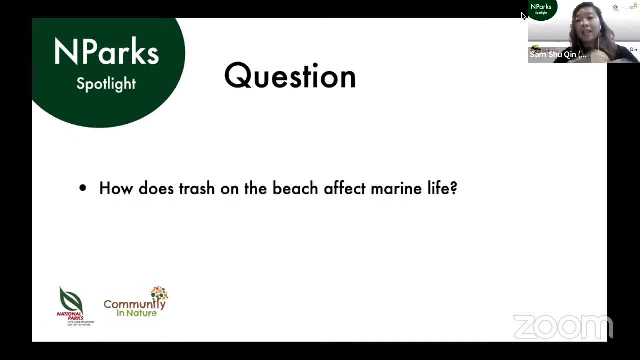 So this is also a problem. We also see a lot of long life nets. Okay, So all these nets. they're able to catch a lot of animals And if they go and float along with the tide, they might end up on the beach. 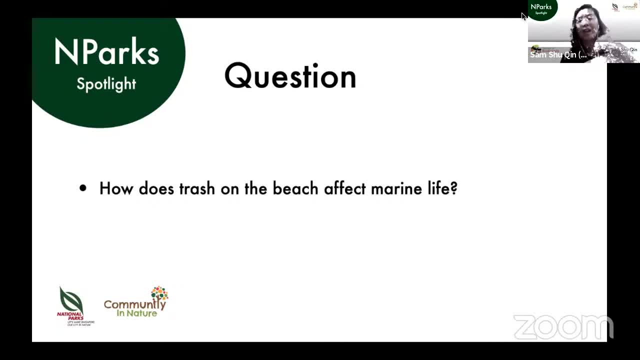 And this will bring a lot of animals that you know. they get tangled with it, So this can be a problem also. So trash on the beach not only affect marine life. they also affect us in terms if they go down the food chain. 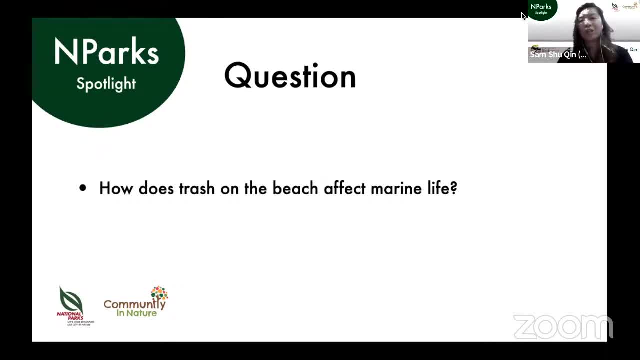 we might end up eating them, And also, if you have trash on the beach, you won't even want to go to the beach to enjoy yourself, right? So it might affect some kind of tourism and our mood also, And also some of them can be quite fragile and sharp. 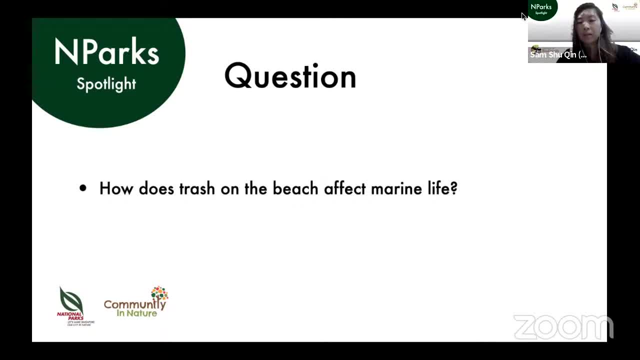 So if they are broken, so it can be quite tricky also. So if you are doing beach cleanup, be careful also. wear covered shoes and do not pick up any sharp stuff. Okay, So you know trash is harmful for marine life. 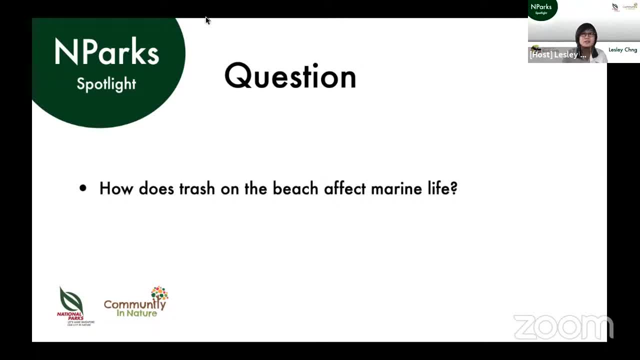 Some animals might mistake it for food, or sometimes it can trap or even hurt the animals. And it also contaminates the marine environment and affects the delicate balance which many of these creatures need to survive. And you know our environment is interconnected At some point. 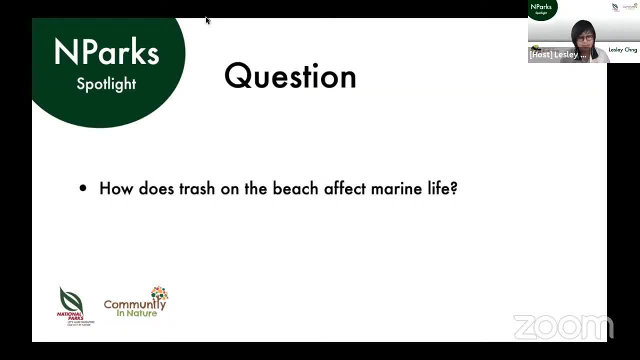 it will come back to affect us as well. So bottom line is: you know, we need to take care of trash responsibly or, even better, try to avoid generating so much trash. Next question: Do I need to be a diver to volunteer? 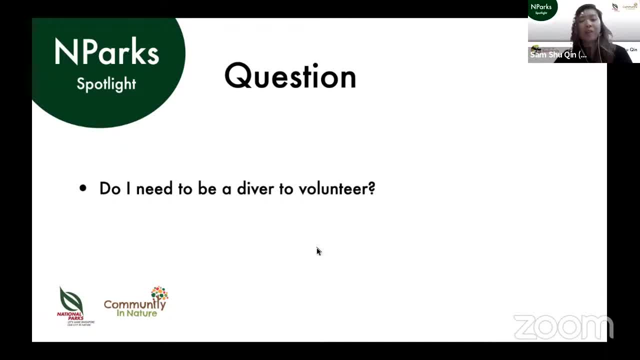 You definitely don't have to, because there are so many groups out there working on different marine conservation causes different habitats, different animals, And there's also a lot of opportunities to volunteer in marine conservation And you can also support this organization in managing like social media. 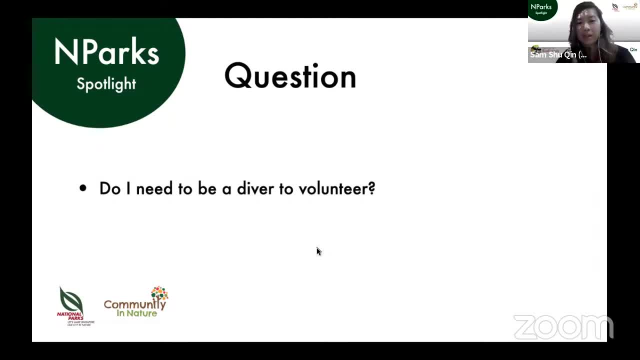 You can also follow them, go on road shows to do some public engagement, talk to the public, sharing the experience. So if you can really talk, this is somewhere that you can go also And also even provide logistical help. So you just need to find a cause. 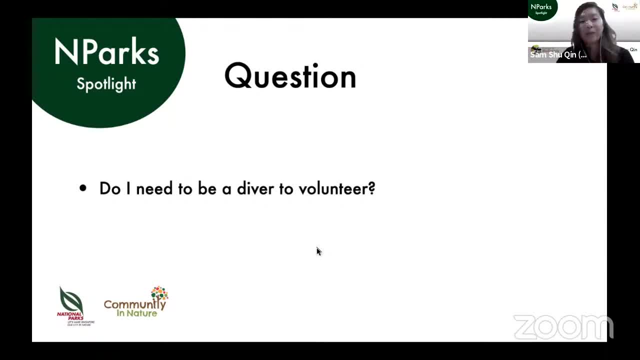 or an animal that you really like, and you start from there. Okay, So I think even during your presentation you talked about how there are different ways to contribute. You know there are some which some people who can do the research, So that one. 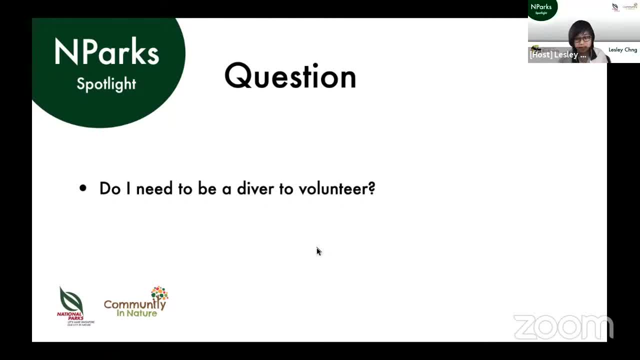 you might need to dive, but there's still other ways, like you know, the beach cleanups and you know helping out on social media, And there's also different. even within the marine environment. there's different habitats which you do not need to be a diver to access. 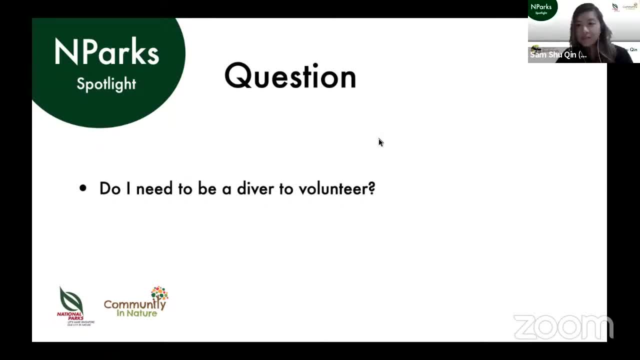 such as the intertidal areas. Okay, So you do not need to be a diver to volunteer, That's true. To add in also: yeah, so you have teams working on mangrove, on seagrass, on the intertidal zone. 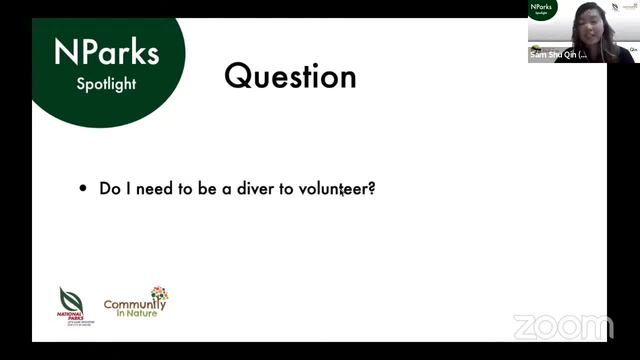 that you don't have to get really, really wet, So it's really accessible to different levels of volunteers. So if you're a diver, there are definitely Hantu bloggers that have our Singapore reef to reach out to if you want to do your part in marine conservation. 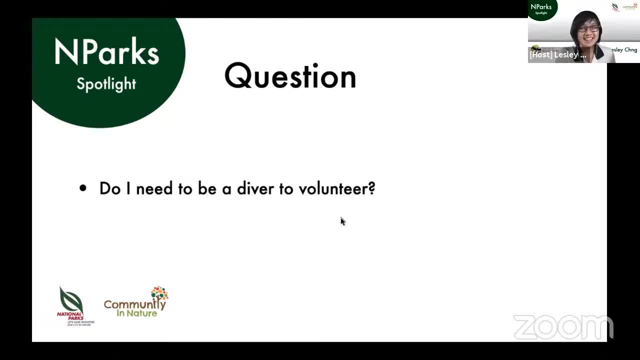 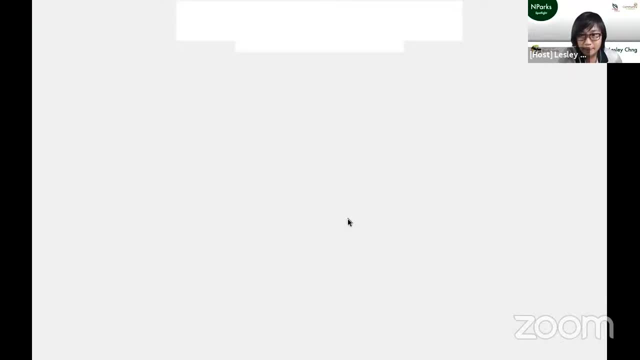 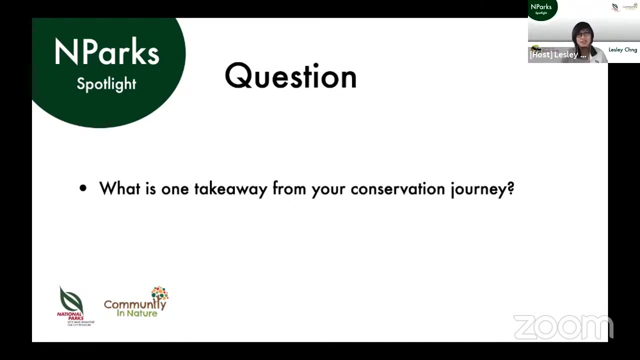 Yep, Many ways that you can contribute. Okay, Next question: Hold on for a moment, Right? Okay, What is one takeaway from your conversation about your conservation journey? So I've learned that you are actually not alone in this journey, So what you have to do is to find your support group. 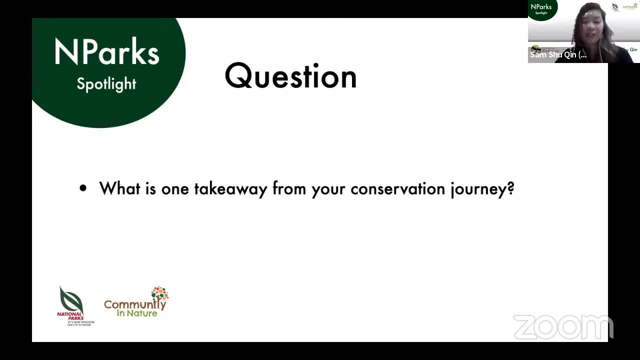 And I'm glad that I found mine. So they have really been supportive throughout the journey and have given me a lot of opportunity to grow as a person and also to grow our Singapore reef as a community. So just don't be afraid to ask questions. 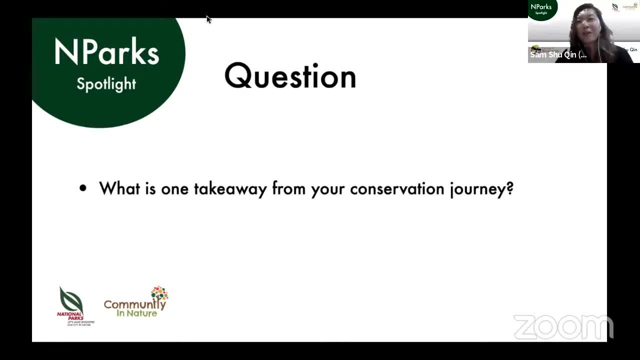 They're all very helpful And all the little things and lessons you take from them will be very, very valuable. So this is what I have. Okay, That's very nice to hear. Like, connecting with people is very important And I think you know. 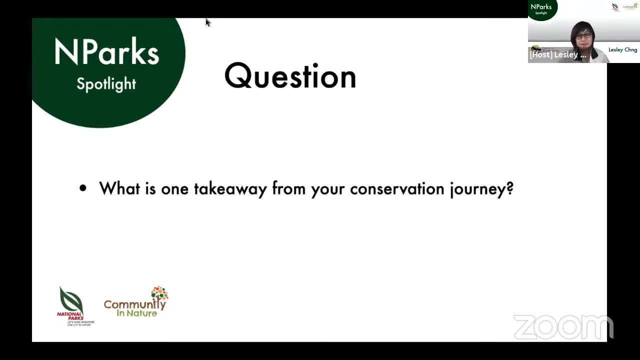 many times during a presentation you did describe the Friends of Marine Park as like a family, So it's really nice to hear that this has become more than just like a cause that you advocate. but having this community that you can rely on, I'm sure it helps keep you going in this scene as well. 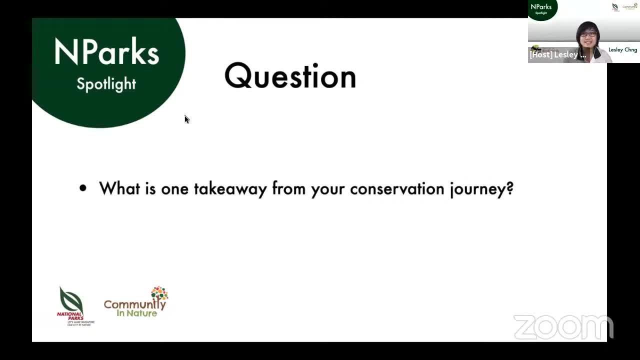 So thank you very much for sharing today The work which your team at Friends of Marine Park I think really exemplifies how multifaceted conservation is. You know you need people from all walks of life. It's really a community effort and everyone can play a part. 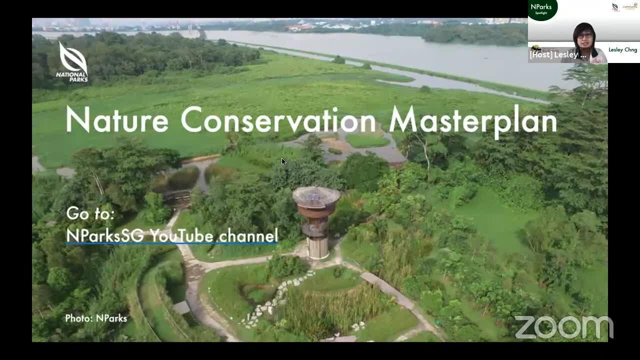 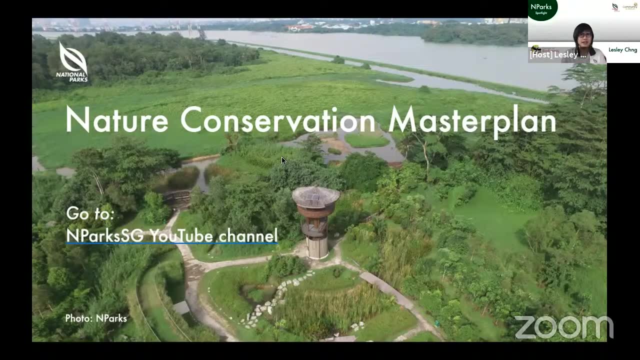 So here at NParks, we recognise ground-led initiatives like Friends of Marine Park as key stakeholders, which is why community engagement is one of the thrusts of NParks Nature Conservation Master Plan, Our systematic approach to conserving our biodiversity and transforming Singapore into a city in nature. 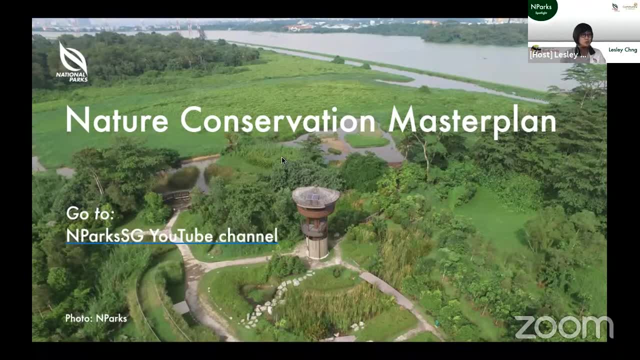 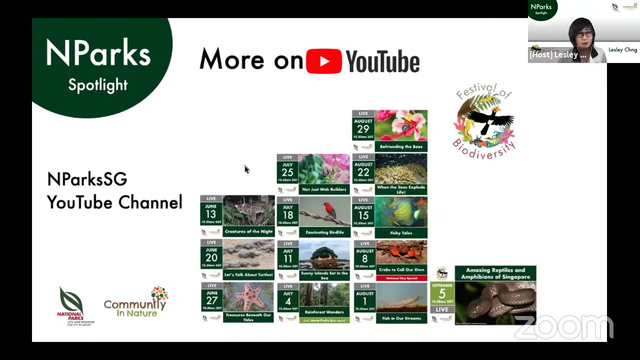 For more information, do check out the links being shared in the Zoom chat or watch our first NParks Spotlight Talk on YouTube. In it, our Group Director, Lim Liang Jim, outlines this plan. On our YouTube channel, you can also catch up on previous sessions of NParks Spotlight. 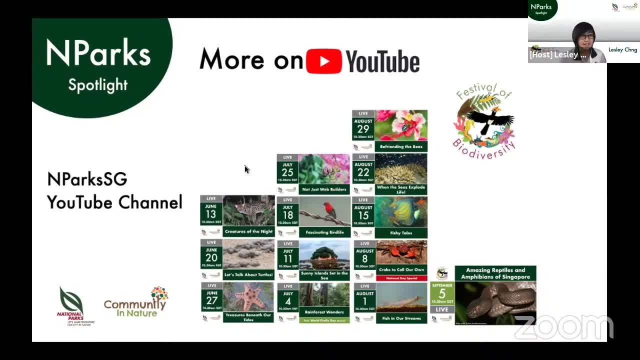 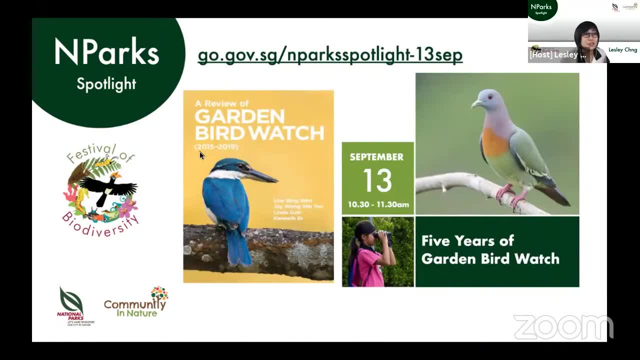 We also have other Festival of Biodiversity activities being live-streamed, so do keep a lookout Now. NParks just released a new book called A Review of Garden Birdwatch, which features observations of birds in our parks and gardens gathered by citizen scientists as part of our Garden Birdwatch programme. 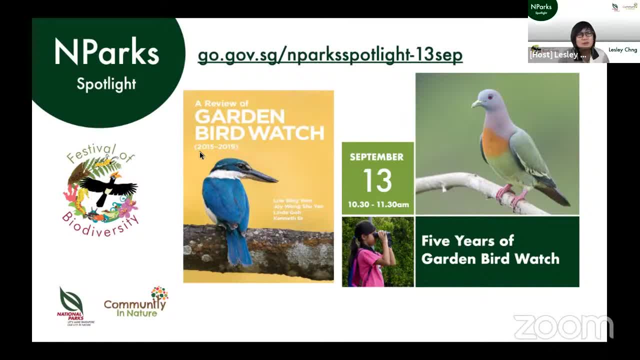 Tomorrow on NParks Spotlight, one of the book's authors, Lo Ping Wen, will be sharing some of the trends and highlights observed. So join us at 10.30 on Zoom or YouTube to find out how our birds have been doing. You can register for the Zoom session at: 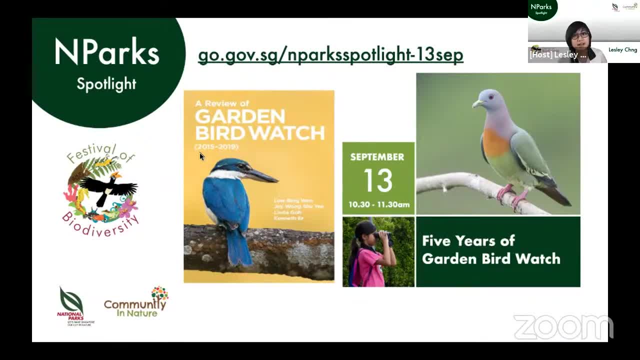 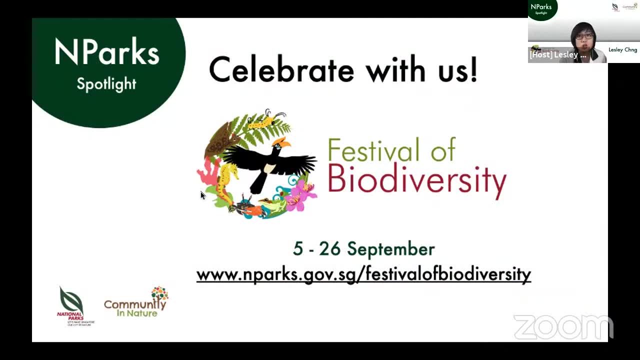 gogovsg slash NParks Spotlight dash 13 September. The registration link for tomorrow's talk will be sent in the chat. And don't forget that we have lots more biodiversity activities for all ages from the 5th to 26th of September. 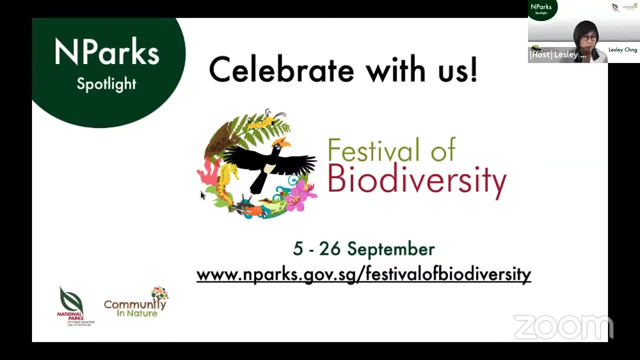 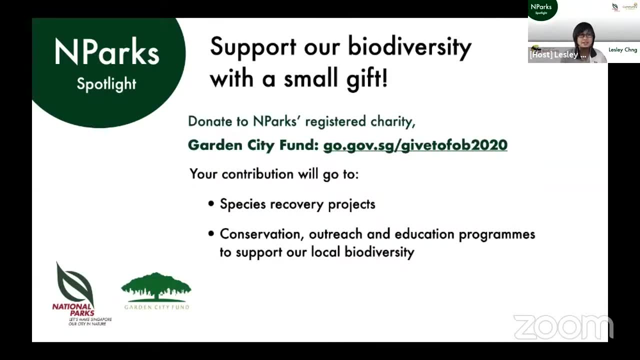 Visit the Festival of Biodiversity webpage for more details. Finally, if you are inspired to support our local biodiversity, we hope you will consider making a donation to NParks registered charity and IPC Garden City Fund. 100% of your contribution will go into species recovery projects.